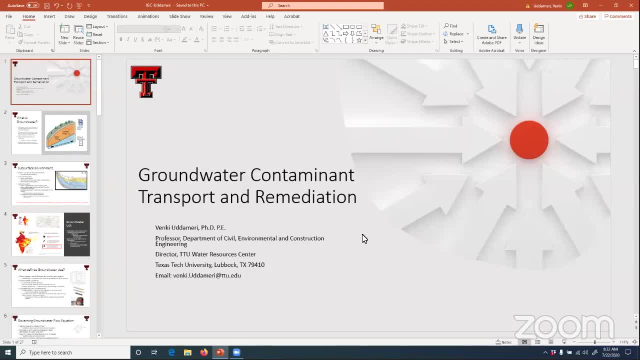 University, where he is also serves as the director of the Texas Tech University Water Resource Center, a university-wide center focused on sustainable water resources problems. He is also an honorary professor of the Faculty of Civil and Environmental Engineering at Jamia Institute of Technology, Ethiopia. 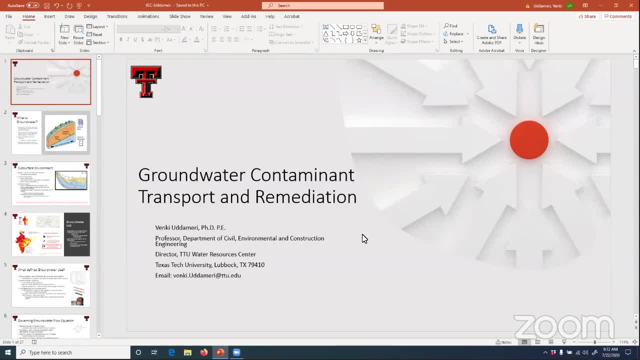 He is currently the editor-in-chief of the Journal of American Water Resources Association, a preeminent journal on multidisciplinary water resources research published by Wheatley InterScience. Prior to joining Texas Technical University in 2012,, Dr Uddamuri was a professor at Texas A&M University, Kingsville, for 11 years. 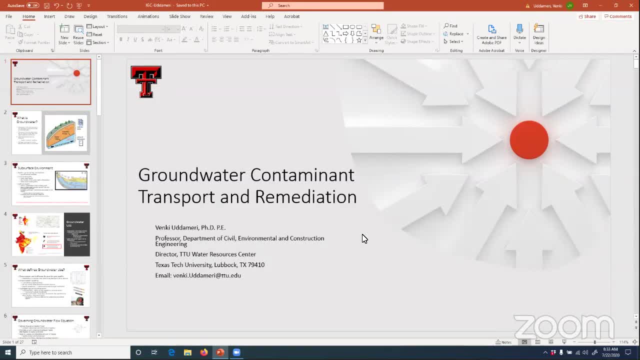 where he is also head. He also founded the National Science Foundation funded Center for Excellence in Science and Technology Research on Environmental Sustainability in Semi-arid Coastal Areas. His primary research interests are in the broad area of water resources, with an emphasis on developing and applying the mathematical modeling techniques to processing water resource problems. 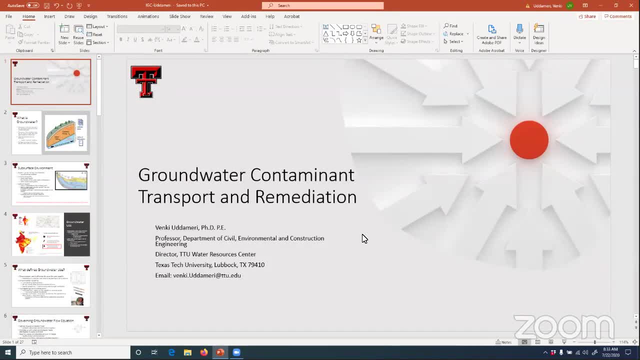 His current focus is on the use of stochastic analysis. He also loves risk assessment methods to assess risk to water systems under climate change, on the use of big data and physics-inspired machine learning methods for sustainable water resources engineering. He has authored over 85 peer-reviewed journal articles and book chapters. 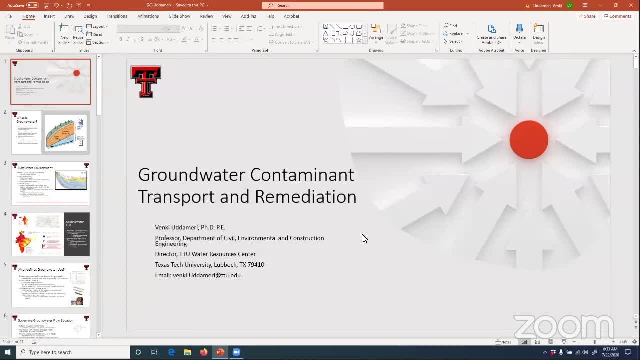 He also has authored two textbooks and is in the process of writing another on water resources planning and management. Dr Uddamuri has conducted research in excess of 18 million and has received funding from a wide range of federal, state, local and international agencies, such as the National Science Foundation, US Department of Agriculture, US Department of Defense, National Oceanic and Atmospheric Administration. 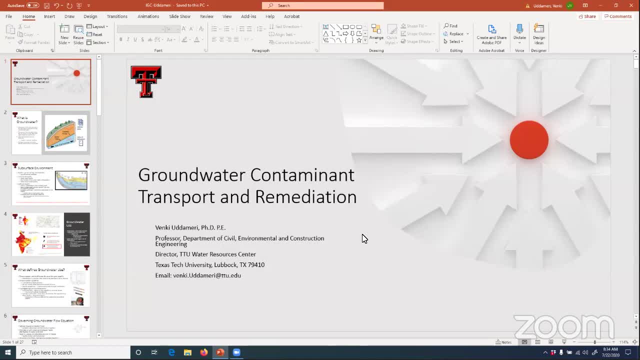 In the year 2016,. he was an invited panelist to discuss national water policy, organized by Office of Science, Technology and Policy of the President Obama's White House. He has made several invited presentations worldwide and recently organized a specialty conference on improving water infrastructure through adaptive resilience. 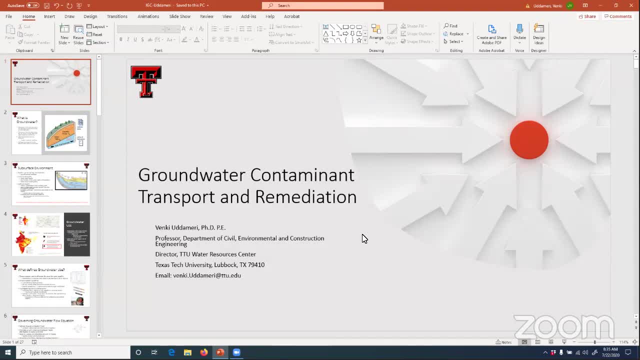 Dr Uddamuri. Venky Uddamuri has taught a broad range of courses at both undergraduate and graduate levels in the area of fluid mechanics engineering, hydrology, surface water, groundwater hydrology, groundwater contamination, transport. He leads the systems thinking initiative within the civil engineering department and has developed a new graduate certification curriculum titled DAS. 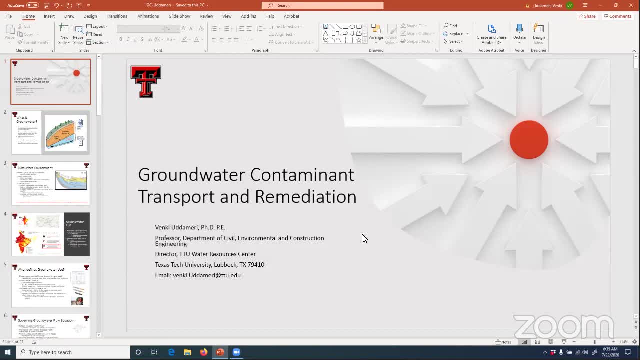 In 2013,. he was invited by the another conse of the project And Dr Uddamuri Back Back. that is GAN network program in the year 2018. so now I am handle the session to Dr Venky Uddamuri, sir, thank you. thank you for that introduction. I hope you all. 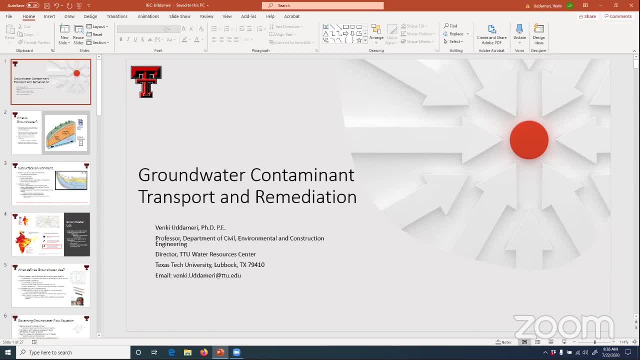 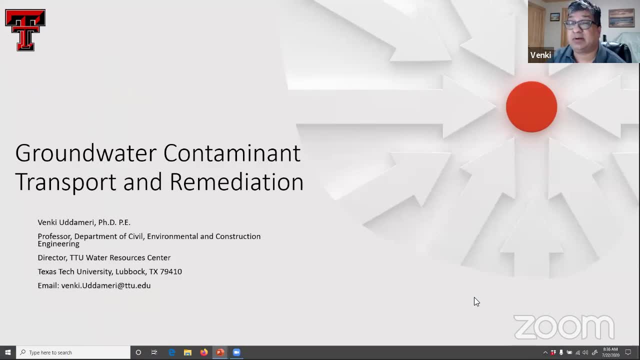 can hear me. well, yes, sir, yeah, great, so I'm going to go ahead and talk today about groundwater contaminant transport and remediation. thank, Dr Ramaroh, for the invitation to give this presentation, so I'm very excited to to be presenting this, and what I'll do is generally give you a broad overview of how do we do. 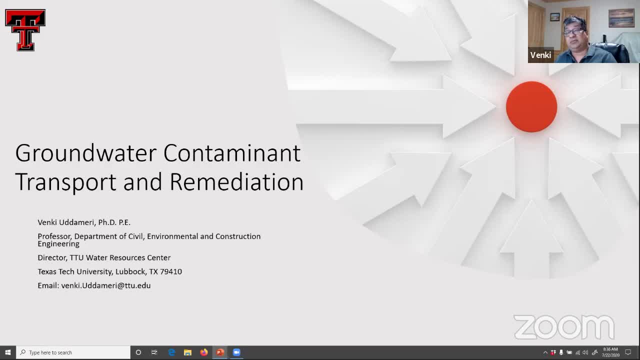 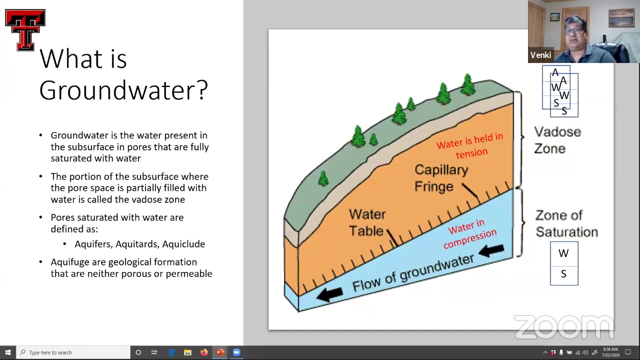 groundwater? what is? what are the various things we do when it comes to groundwater, contaminant transport, modeling, as well as remediation? so, again, you know, I try to keep it as brief as possible so that we'll have time for questions and answers in the end. so let me start off by talking about what is groundwater. you probably all know what. 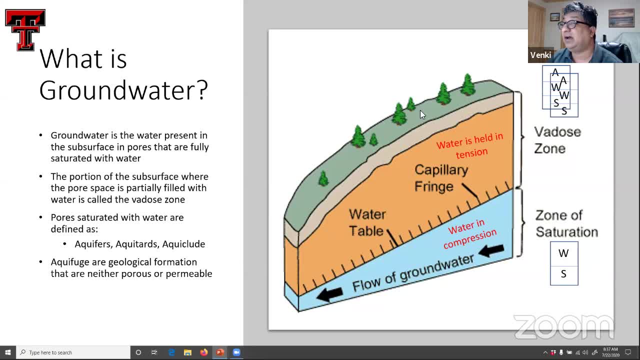 groundwater is. so we have a surface environment and then down below that surface environment is our subsurface environment, and our subsurface environment can be broadly categorized into two, two zones or two areas. okay, the one, which is the shallow environment, is what we refer to as the vedo zone or the partially saturated zone, because, if you go, 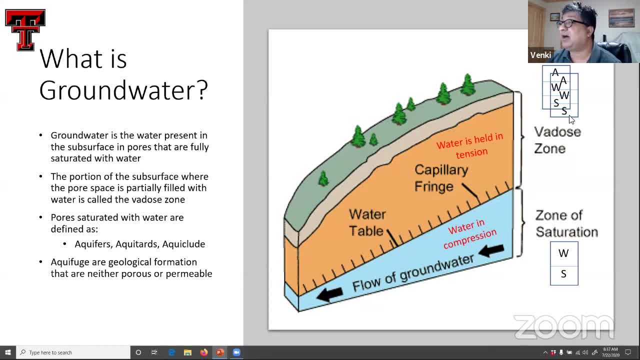 back and look at the phase diagram. here you have air, water and soil. So there are three phases in this subsurface beta zone. And down below there is an area which is demarcated by the water table And that is the zone of saturation. So you have, the pores are fully saturated with water. So 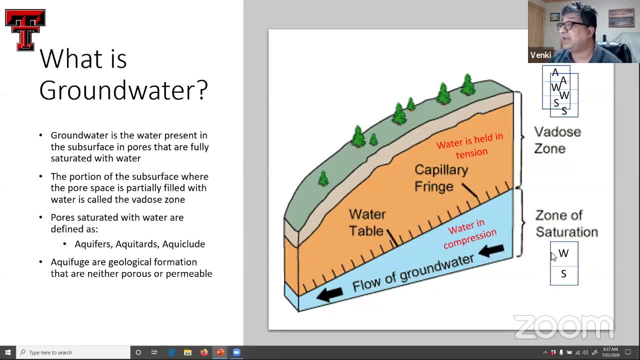 again, if you look at your basic phase diagram, there are two phases here: the waters which fill up the pore spaces and then the solid matrix which holds that down, which causes that pore spaces. So if you look at the beta zone, the water is held in tension because you have two fluids. 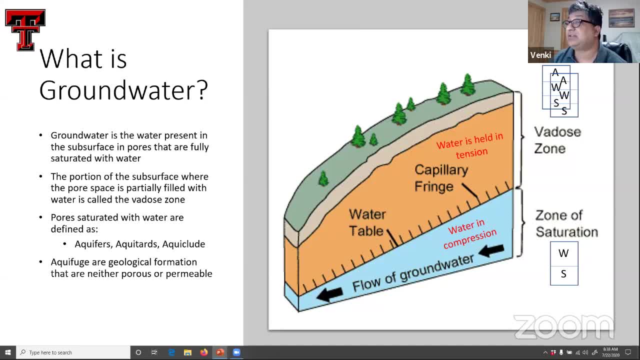 air and water competing for that pore space, So they're trying to push each other out. So that's why the water is held under tension. So it's the surface tension that holds that water And the water is essentially under compression because the pores push the water out, So the water is. 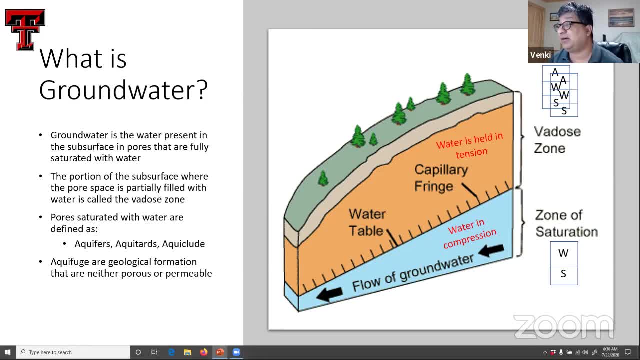 pushed at water. as the, as the pores are fully saturated with water, the rock matrix is pushing that water, which causes the flow of groundwater. So when we talk about groundwater, we are only talking about water that's below this water table, or in, or in or in subsurface environments, where 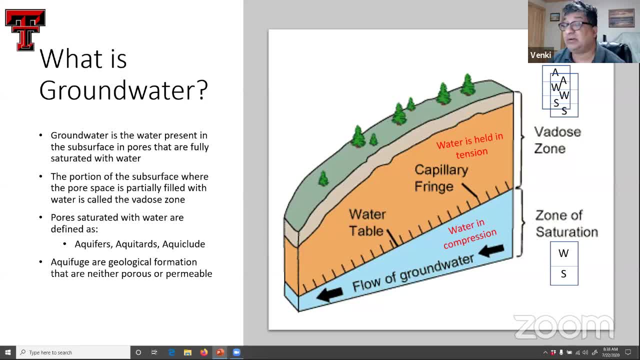 the pores are fully saturated with water, So there are many types of groundwater environments. aquifers are basically units that produce large quantities of water, So that's of interest to us. If we want to develop a water supply project, we typically look for aquifers, because there's a sufficient amount of water of. 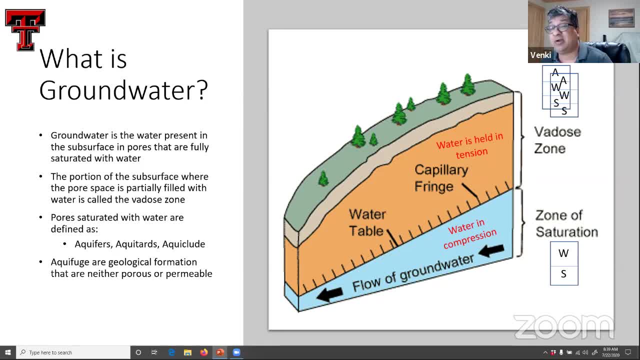 good quality usually, as well as well as sufficient amount of quantity. But you can have other types of geological formations then with the aquitards and the aquifluids. Aquitards, as their name comes, essentially are they. the water can move through them, but it moves very slowly, So 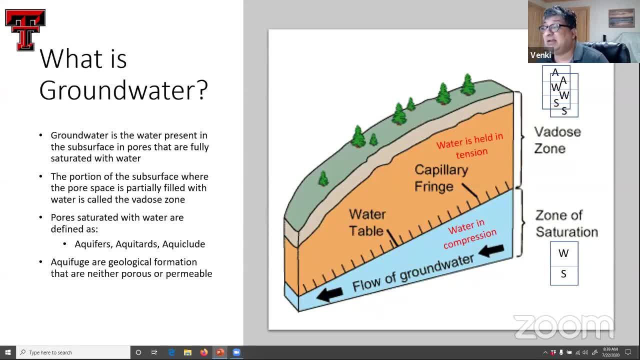 in terms of water supply, we really don't develop sources in aquitards, But when it comes to contaminant transport, aquitards play a very big role, because the contaminants can get trapped in aquitards and sit there for years and years and years and sometimes centuries, and slowly leach. 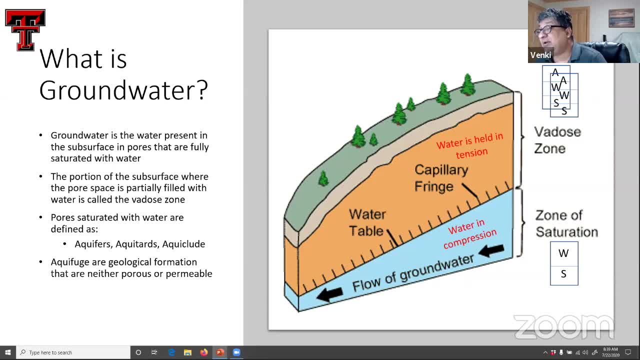 into the underlying aquifers, So so. so, when we, when we deal with contaminant transport, aquitards play a very big role as well. Aquifluids, on the other hand, have water, but they don't really transmit water. But again, from a contaminant transport perspective, 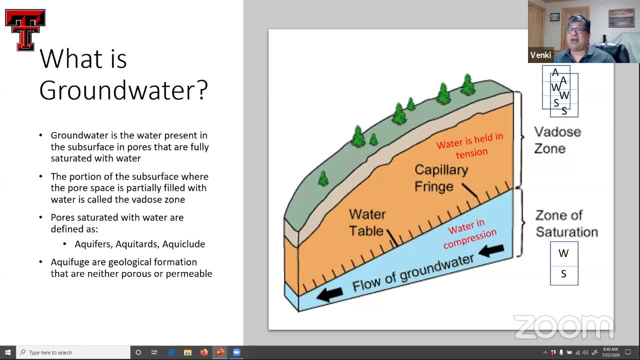 they're very important because the contaminants can get trapped into aquifluids and then diffuse out very slowly over a very long period of time, causing contamination. So so when we talk about water supply projects typically get interested in aquifers, When we talk about contaminant. 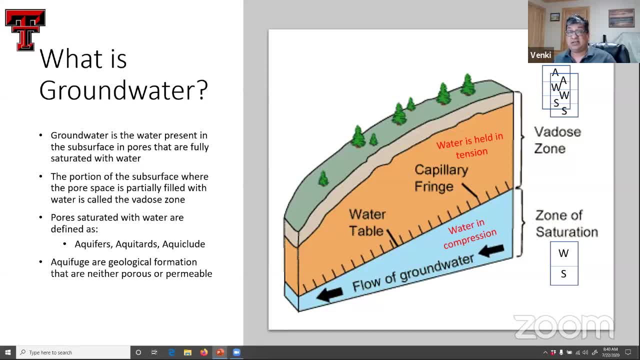 transport issues. we look at aquifers, aquitards and aquifluids. Of course you also have aquifuges, which are geological formations. So you can see here you can see that there's a lot of geological formations that are neither porous nor permeable, So we don't pay much attention to. 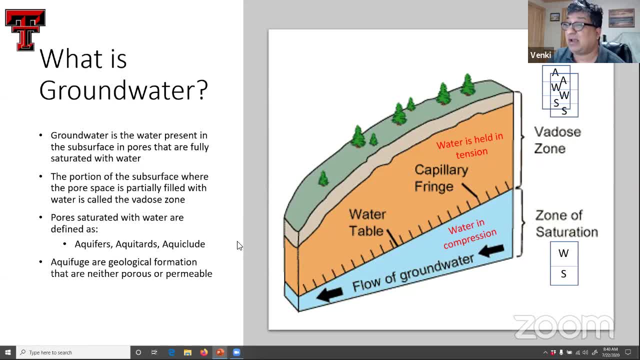 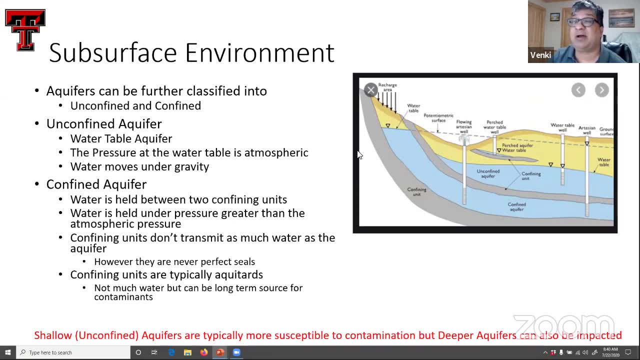 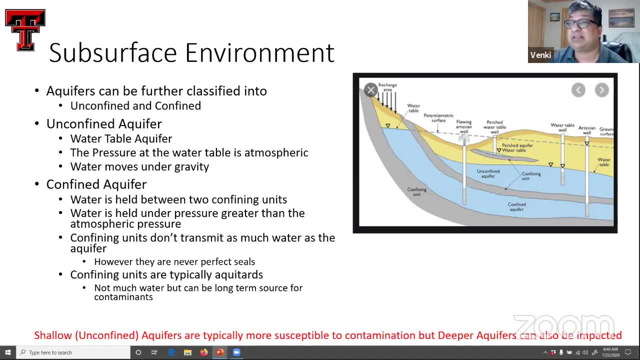 and the confined aquifers. You probably have talked about this in your geotech classes as well. So, and essentially, an unconfined aquifer is characterized by a water table, And this water table, or the surface of that water table, is open to atmospheric pressure. So there, 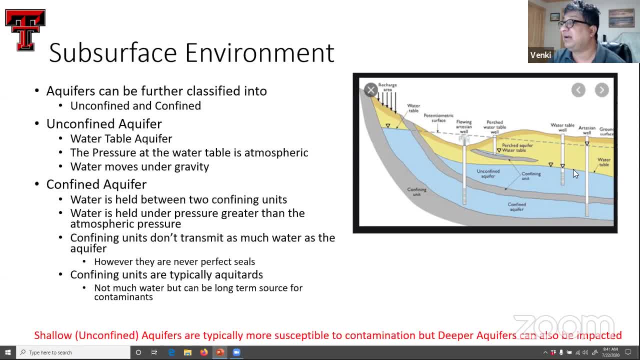 is atmospheric pressure acting on this or roughly atmospheric pressure acting on that water, on the surface of the water table, And, of course, the pressure increases as we go down in depth. And a confined aquifer is an aquifer that is confined between two confining layers, usually of very low permeability. Typically these are rock formations or these could be clay formations. 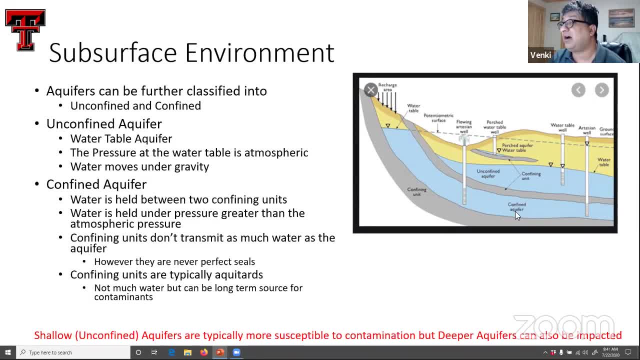 So they basically confine the water or the aquifer that's in between And, as a result, the water is under pressure because it has an overburden pressure from the top that puts it under a pressure higher than the atmospheric pressure. So typically, if you put a well in the right place in a confined aquifer, you can get what's called an artesian well or a well that flows by itself, for saving you a lot of energy. 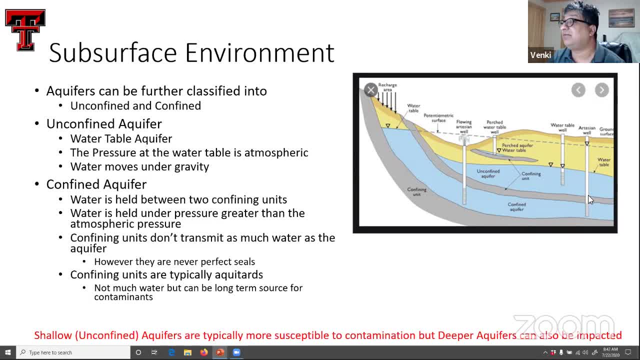 But in general, when we put a well, When we put a well in a confined aquifer, the water level rises much above that confined aquifer And that is what is what we call an artesian well. So that's because the pressure is released. you know, the pressure here is atmospheric and the pressure here is some positive pressure. 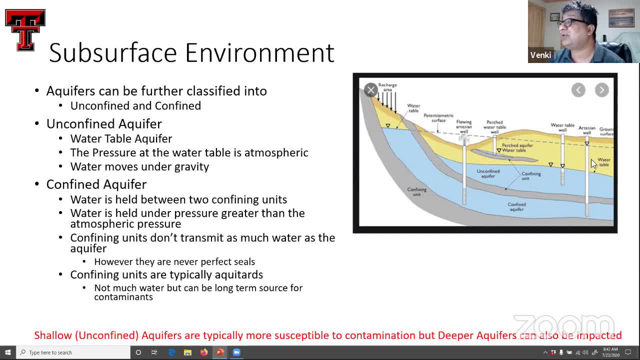 So the water moves from higher pressure to lower pressure until it equilibrates and causes the water in that well to move much higher than where the aquifer actually is, Whereas the water table is where the water is, So that's where it defines the pressure, in an unconfined formation. 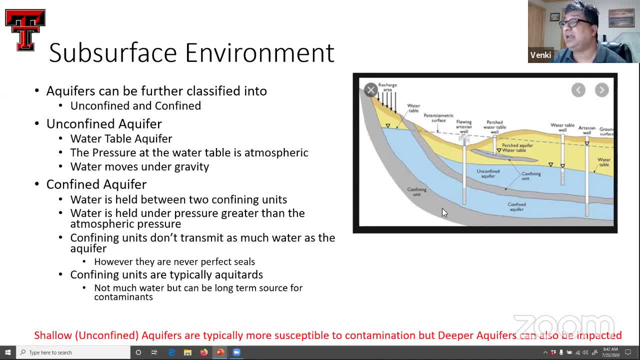 Even though we talk about these confining units, they are strictly not impermeable. We, for some purposes of analysis, we assume this to be impermeable but in reality these confining units typically are aquitards. So if you have a contamination present in that aquitard then it can slowly leach in and leak into these confined formations. 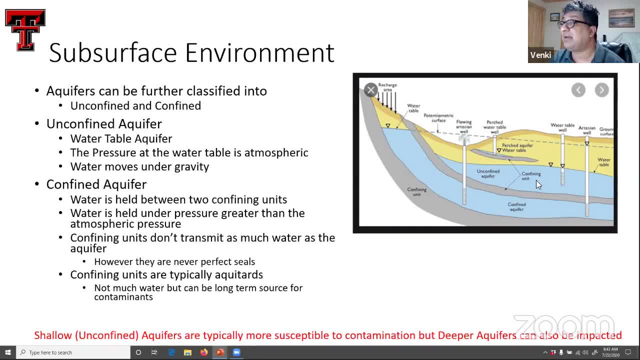 Or it can move up into the unconfined aquifers and contaminate the aquifers. Another type of aquifer that's very common in bedrock conditions, like in India, are the perched aquifers. These are small sand deposits that are very shallow and they usually supply water to dug wells or very shallow wells. 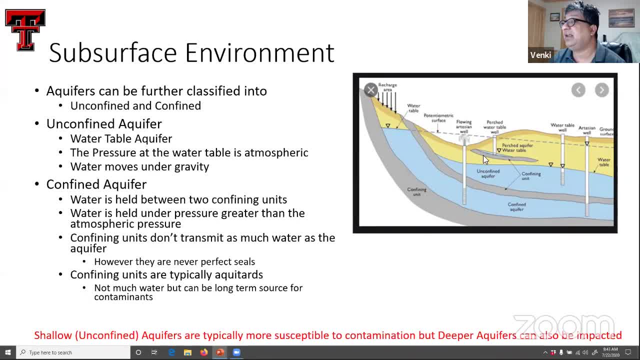 So these are generally under perched conditions. So there's a playland or something that will cause water to store and create an aquifer, you know, a very small aquifer that cannot be exploited for very large water uses but can be used for smaller demands, to meet smaller demands as well. 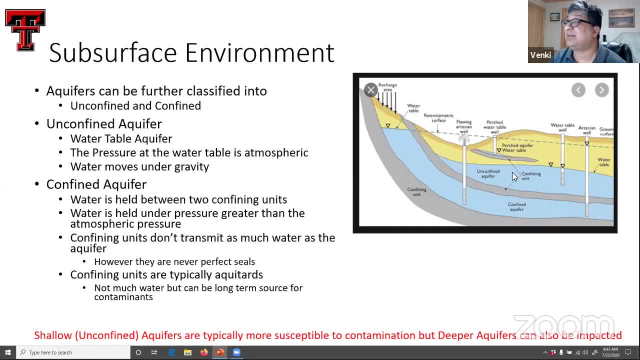 So typically, the shallower the aquifer is, the more susceptible it is to contamination, because contamination usually happens at the surface. We do something in the surface that causes contamination, And so the perched aquifer or the unconfined aquifers are effective. 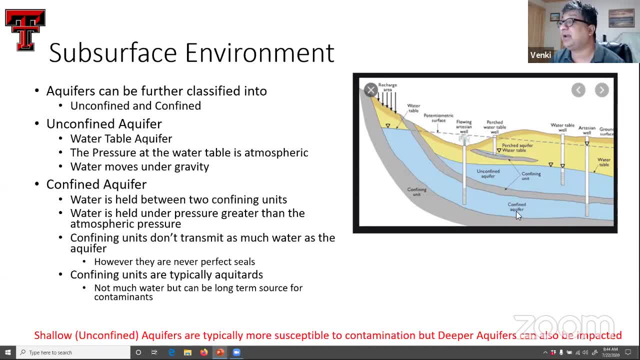 That doesn't mean that the confined aquifers are not affected by contamination. They can also be affected, as I said, like if a contaminant gets into this aquitard, it can serve as a very long source of contamination. So let's talk about groundwater a little bit. 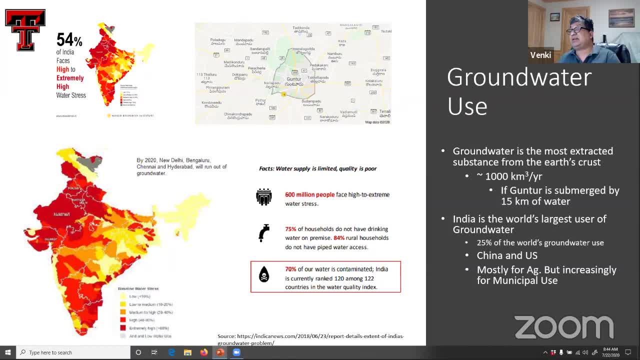 Groundwater is the most extracted substance in the earth's crust. Typically, we use about a thousand kilometer cube per year of water. That's a lot of water. So just to give you some perspective, The city of Gujarat is about 60 square miles, or 60 kilometers in area. 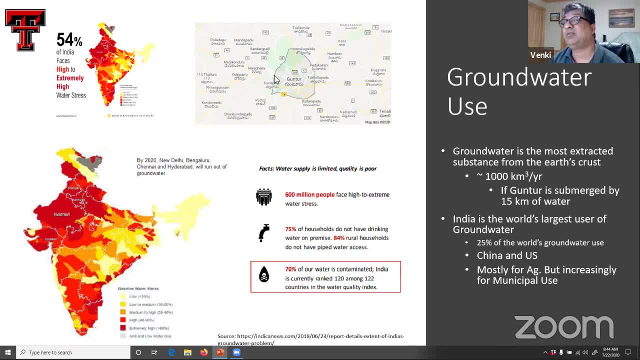 So if I have a head of about 15 kilometers of water on top of it, that is the amount of water that would be used. Imagine the water on top of this area extending about 15 kilometers all the way up into the atmosphere, And that would be the amount of water that we use. 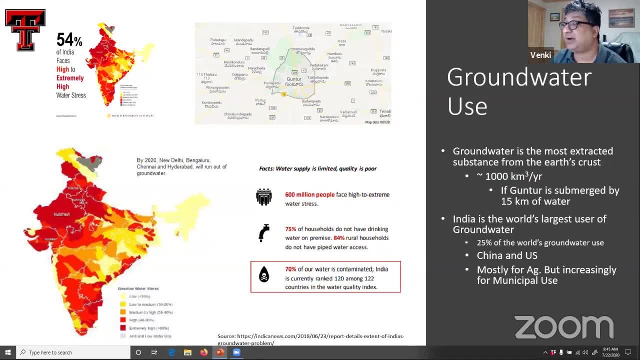 So we use a lot of water, And India, of course, is the largest user of groundwater. About 25% of the world's groundwater use happens in India. Of course, in China and the US are the two other larger users of water. 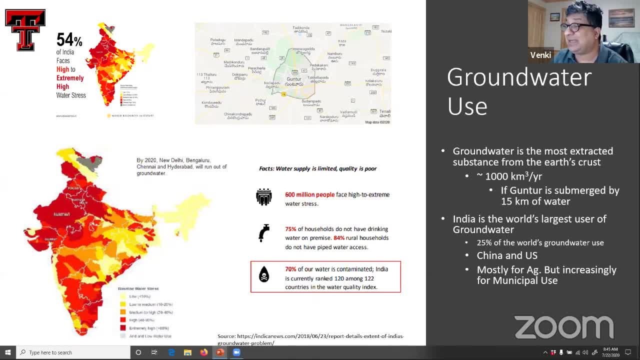 And mostly water is used for ag, but increasingly this is being exploited for municipal use. Everybody kind of knew about what happened last year when Chennai ran out of water, So there is scarcity of water both in terms of the quantity of water but also in terms of the amount of water. 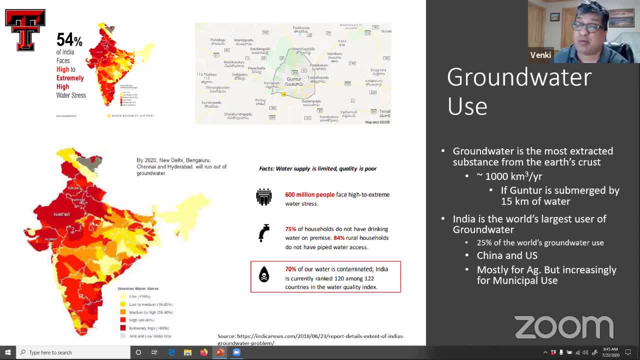 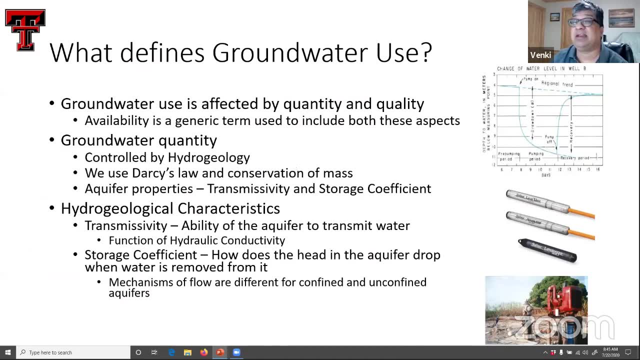 So there is scarcity of water, both in terms of the quantity of water but also in terms of the quantity of water. So there is scarcity of water, but also in terms of the quantity of water. So both these issues are extremely important in a place like India. 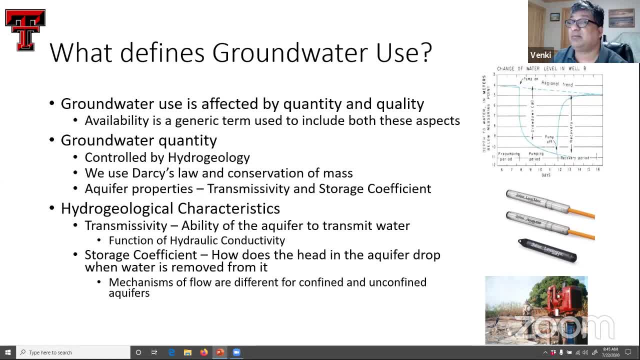 So what defines groundwater use? So when can we put groundwater to use? Groundwater is a resource. We want to use it. Groundwater use is affected by quantity and quality, So we generally use the word water availability as a catch-all term, like as something that captures both the quantity and quality. 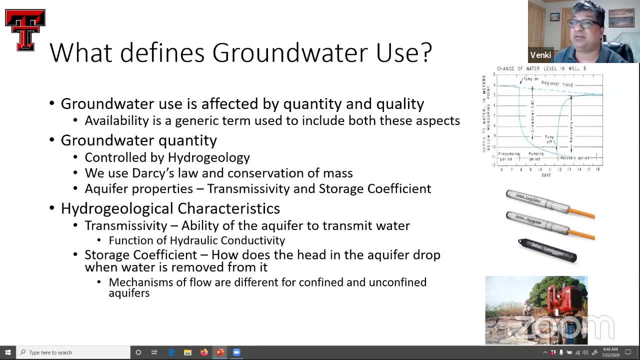 When it comes to quantity, it's largely controlled by hydrogeology. We model groundwater systems using Darcy's law and conservation of mass. Again, you must have studied Darcy's law either in your hydrology or in your geotech classes. 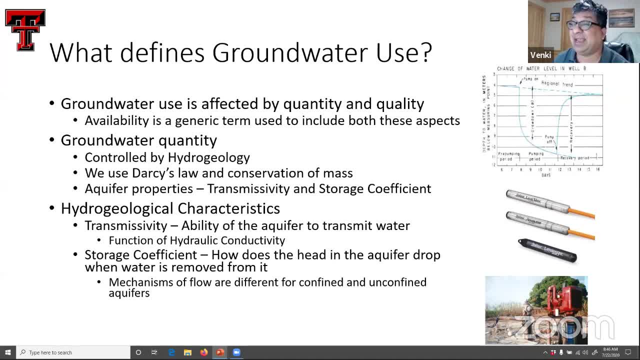 And we need aquifer properties like the aquifer transmissivity and storage coefficients. Those are the two basic properties associated with any aquifer, or the hydrogeological characteristics of the aquifer. So transmissivity, briefly, is the ability of the aquifer to transmit water. 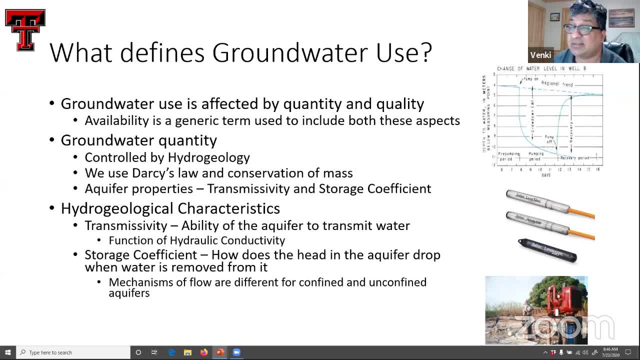 It is the hydraulic conductivity times, the thickness of the aquifer, thickness of the saturated layer in our confined formations, Storage coefficients. this defines how much head, how much of a hydraulic head drop do we get if we remove a certain amount of water over a unit cross-sectional area. 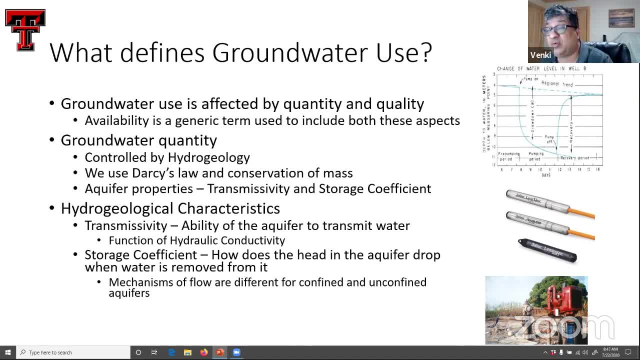 So storage coefficient. water is driven and drained by different mechanisms depending on whether you're in unconfined aquifer or in a confined aquifer. In unconfined aquifer, water is drained due to gravity, So you use the term specific yield. 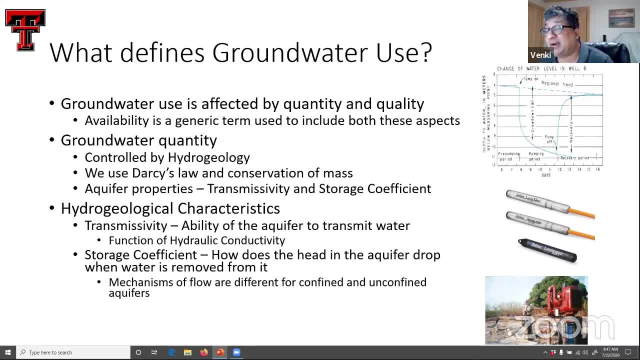 or what is called as the drainable porosity, of the amount of water that can be removed under the influence of gravity. In confined formations, the water is under pressure, So it's really the compression and expansion of that water that causes the water to move out. 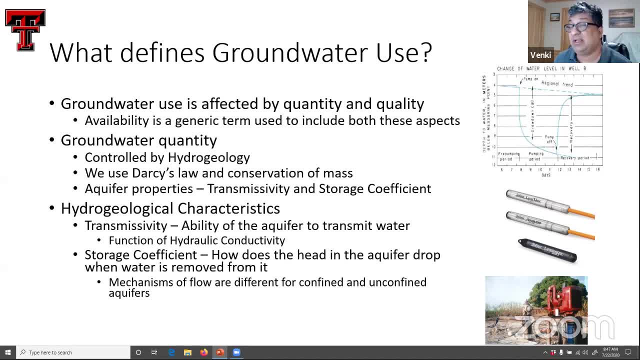 So it's really the compression and expansion of that water that causes the water to move out. So it's really the compression and expansion of that water that causes the water to move out. So the compression of the aquifer matrix and the compression of the water itself. 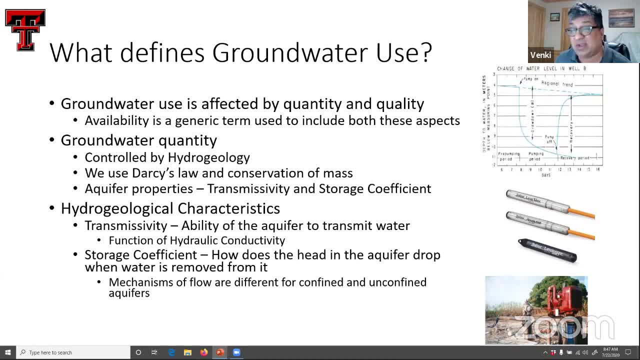 is what causes the water to be expelled out of that system. So we use the word storage coefficient. Storage coefficient is more a catch-all term, a more genetic term that says how much of a hydraulic head drop do we see over the cross-sectional area? 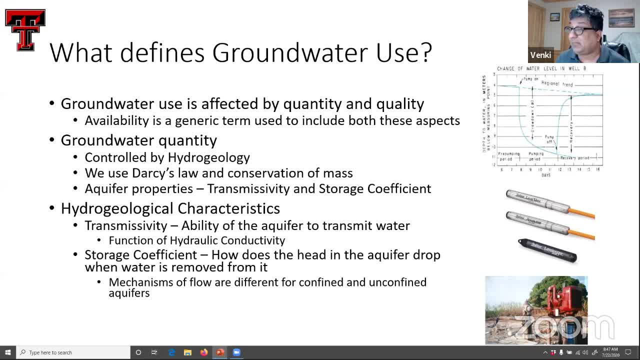 for a given amount of water that we remove. So one of the things to get these information, we do water quality pumping tests. So we drill wells and then start pumping water, So then we see how the water level drops over the period of time. 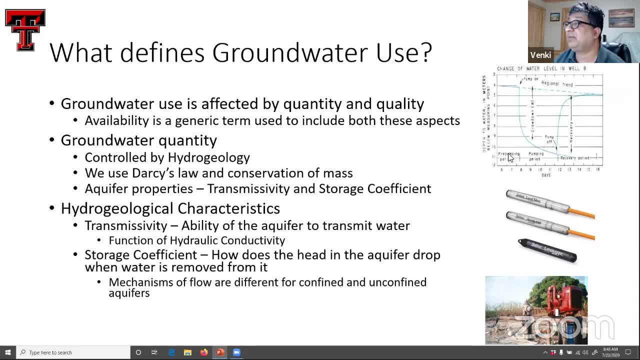 And then we tend to equilibrated for a while, which is called the pre-pumping period, And then we pump so that the water comes down, and then we stop pumping at a time and see how the water recovers back, Of course, as we pump water. 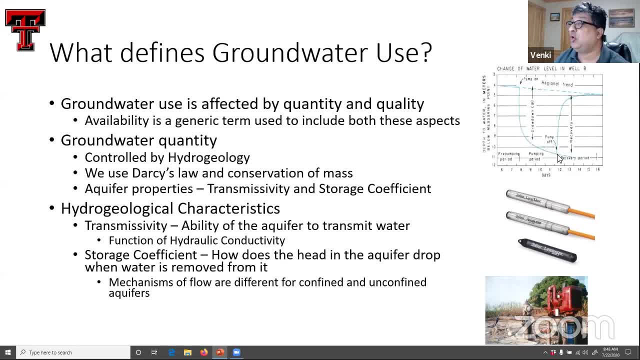 the hydraulic head drops in the dock. of course, locally, the well at this point in time has a lower head compared to the surrounding area, so so the water starts to flow towards the well, and that process is called recovery, and it tends to get back to some equilibrium, uh, sometime later. so so typically we do a drawdown test and a recovery. 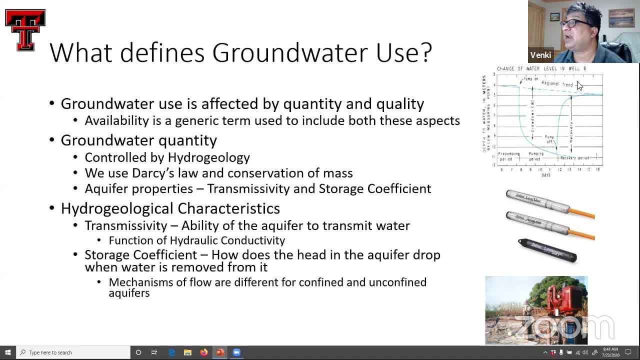 test. uh, one phase where we are pumping and another phase where we are not pumping and we try to get water. these experiments, uh, become somewhat easier over the years, especially over the last 10 years or so. uh, we have started getting really good pressure transducers or water level loggers. 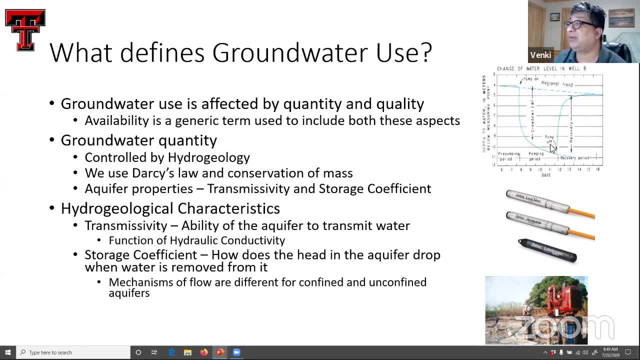 that can required water level drops at fairly quick intervals: uh about, uh a second, or even, like you know, uh, 10 milliseconds or 15 milliseconds. we can do it very reliably these days and that has improved our ability to get these properties- the france facility and the storage coefficients, and again, 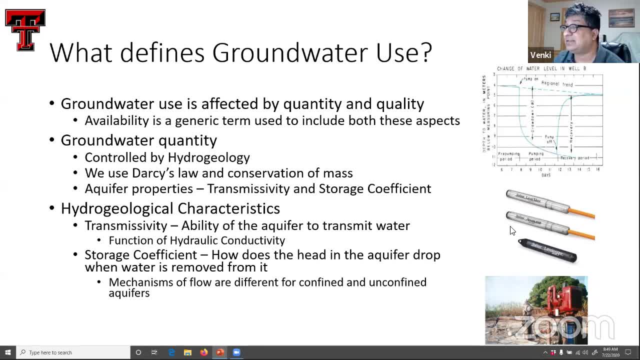 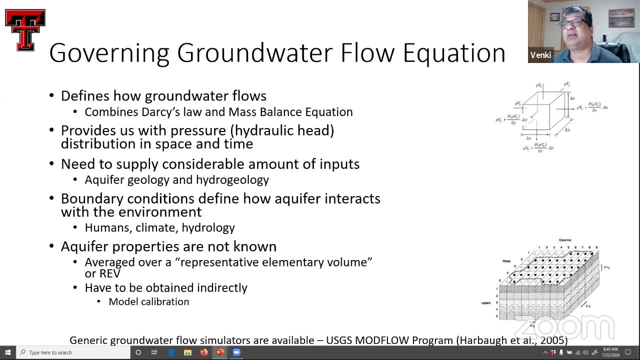 i show you some different types of logging devices, so pressure transducers that we typically install in a well when we do a pumping test to get these characteristics. so once we get those values, we need some sort of a model to describe our groundwater flow, and that comes from what's called as the governing groundwater flow equation. 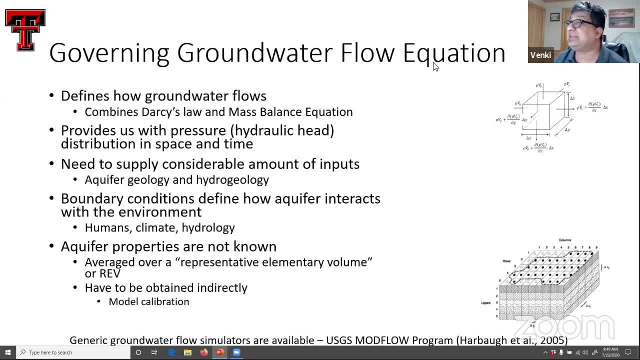 what this groundwater flow equation essentially does is. it takes a small piece of your aquifer and let's call it the representative elementary volume. so it's got an x direction, a y direction, and then it assumes that the water flows in and flows out along all these different directions. 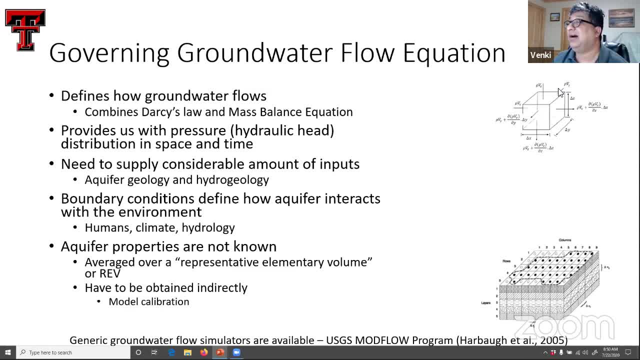 and then uses darcy's law to write the movement of water in and out of that system, and then and then it integrates that over the domain of interest. So that's how we develop the groundwater and groundwater flow equation. To solve this equation we usually will have to solve it numerically, So we grid this. 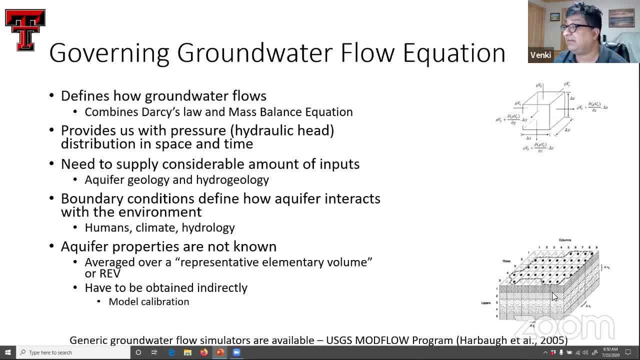 cross-sectional area, both in the horizontal and vertical direction, So you have different layers of geologic formations and then the cross-sectional area of interest to us, So we may have some areas which are inactive, which we turn off, and then, so that we can, 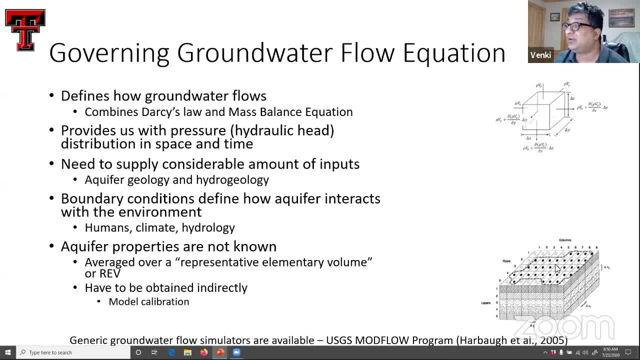 model these irregular boundaries, And then, for each of these cells we have to give: what is the transmissibility, what's the storage coefficient, what are the initial conditions? what happens at these boundaries, like if they're pumping, if they're recharged from the atmosphere? all these 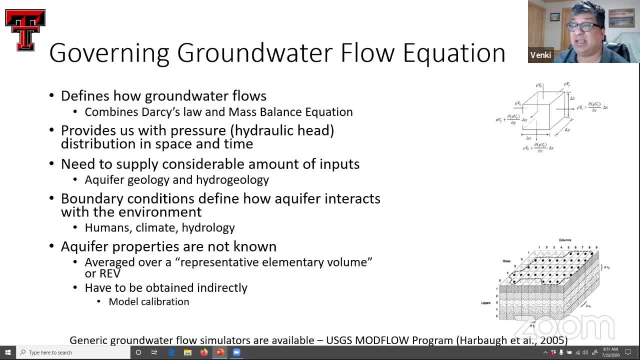 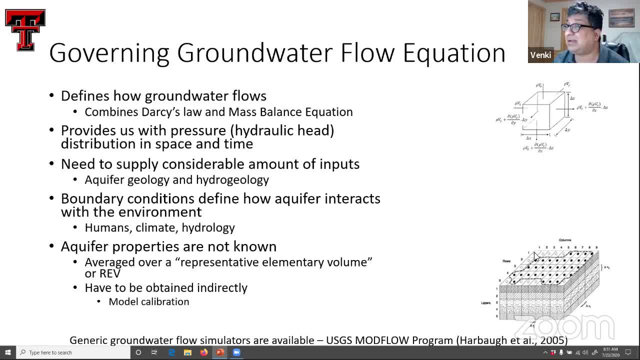 The reason why we have groundwater systems and groundwater flow equations is that we are actually writing the equations at a macroscopic scale. So if we look at the scale of this representative elementary volume, that's sometimes a square mile. And if I'm doing a very large model, we've done some models where we have modeled aquifers in 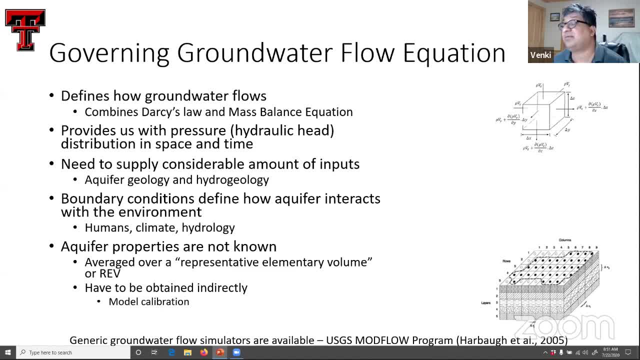 Texas. We have modeled the Ogallala Aquifer, which is the largest aquifer in the US. that actually spreads over eight different states. It's a very large aquifer system. The representative elementary volume in that case is about five square miles or something like that. 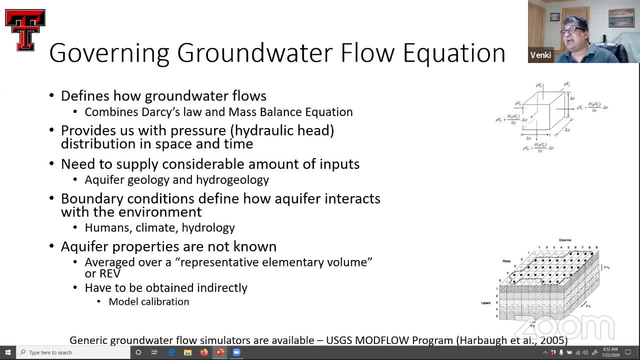 so fairly large systems. So there are many different types of soils. when you get a fairly large chunk of that volume of soil, If you take a core that size, you're going to see many different soils of very different grain sizes. So what happens is: 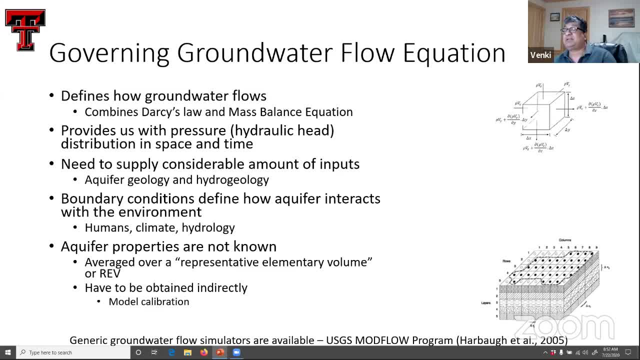 the hydraulic conductivity of the storage coefficients that we are defining is an average over that entire representative elementary volume. So you all know that we cannot measure the average directly. So if I want to say what is the average score in your class, I have to individually know what the individual scores are to get an average. 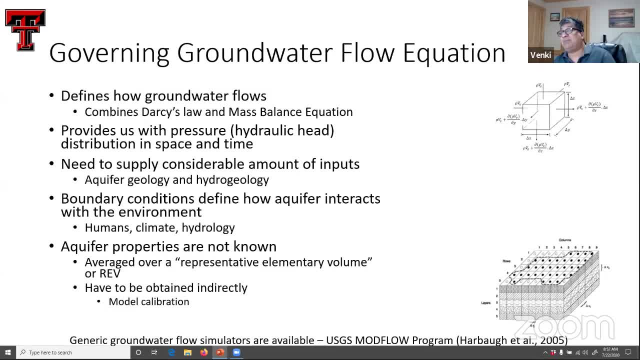 score. I can't just go measure the average without measuring the individual conductivity. So what happens is we have a lot of different models that we have to indirectly obtain these values, So that process is called as model calibration. So what we do in model calibration is we measure groundwater levels. 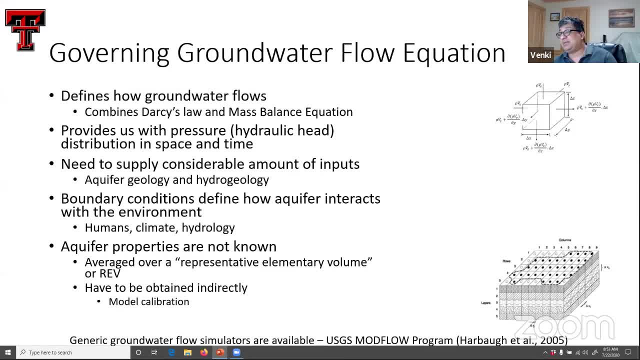 because they're easy to measure. but we really cannot get the hydraulic conductivity or the storage coefficients because we have to use another model to get it, because it's an average property. So we go back and say let's match those water levels to the wells where we have and try to estimate what the hydraulic conductivity is. 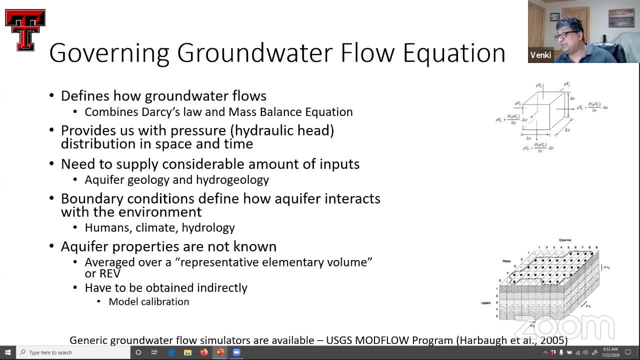 So that's a very simple model: What the hydraulic conductivity is, what the storage coefficient is, what some of the other parameters are, sometimes the boundary conditions and fluxes associated with the boundary conditions. So that process where we are running the model backwards to get the inputs rather than supplying. 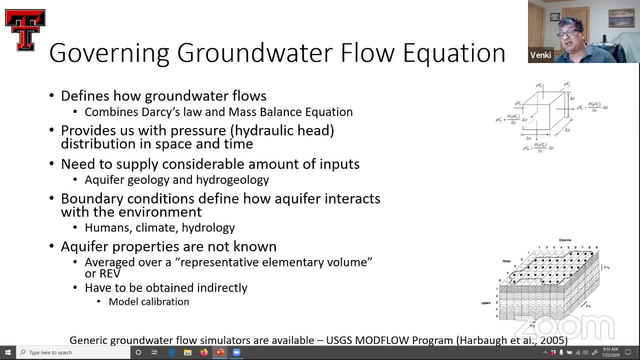 the inputs and getting an output is called model calibration. And model calibration becomes very important- And it's a very challenging problem in groundwater because there is really no unique mathematical solution when we run the model backwards. So we're running the model forward where we supply inputs and estimate our hydraulic heads. There's a lot easier problem. 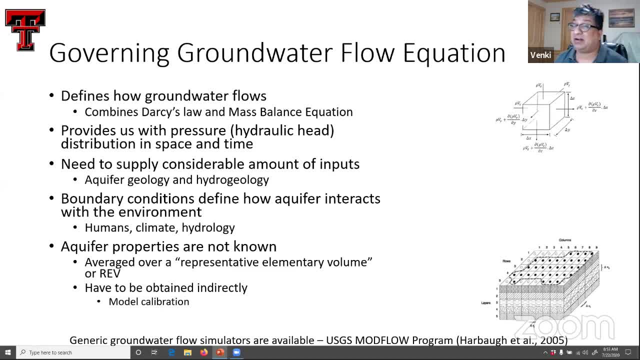 to solve than taking the hydraulic heads and trying to back up what the aquifer parameters are. But we have to do that, otherwise we really cannot calibrate these models. So over the years we've had some generic groundwater flow simulators. The USGS Smart Flow is a very popular program. 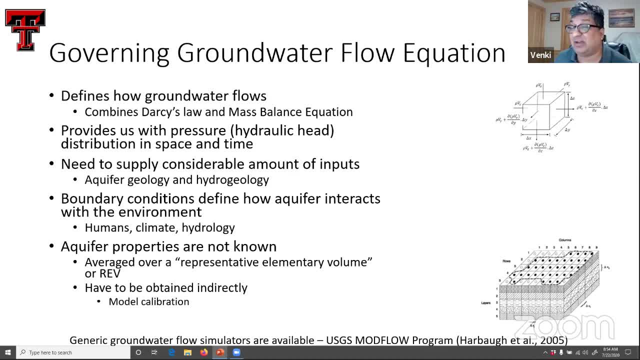 It's an industry standard program. These days, we generally use it instead of writing our own code. But when I started getting into this business in the early 90s, Smart Flow was there, but it was just getting started, So a lot of groundwater modeling involved writing code and 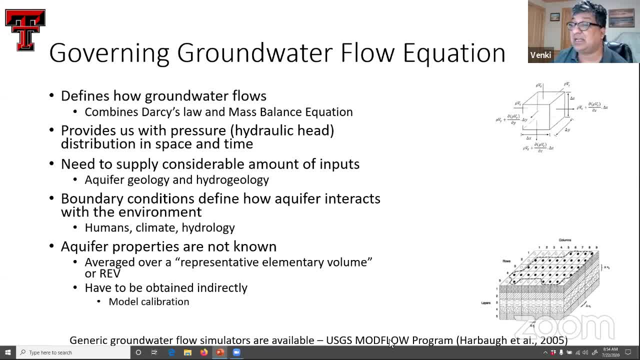 writing these equations and following these equations, But these days we have some really good codes to help out with the simulation, So putting these models together is a lot easier now than it was, at least from a numerical standpoint, But it's still challenging in the sense that 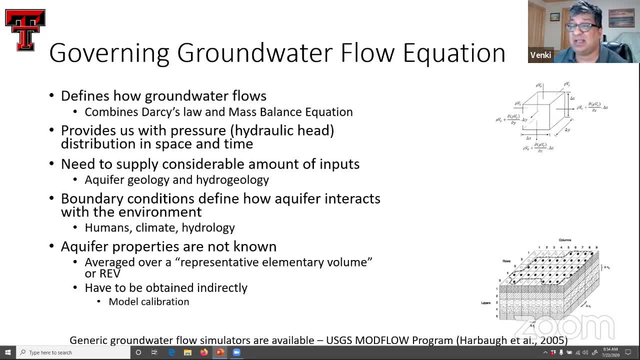 we have to get data from many different places and we have to deal with a lot of uncertainty when we say where does this geologic formation really start and where does it really end, And getting that information from spotty data or from cores or soil bores. 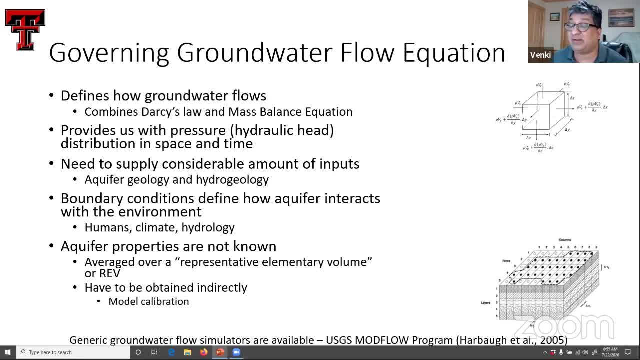 and then extrapolating over a very large distance or interpolating over a very large distance adds a lot of uncertainty to it. that has to be dealt with as we do this modeling process. But that's the flow part of the groundwater equation. So we are just saying we're not looking at any. 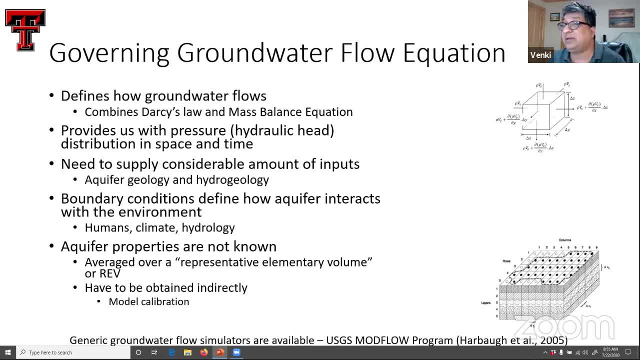 chemicals or any other constituents in that water. We are simply saying how does the water move? And the output of such a flow model would be pressures at all these locations. And of course you know that water moves from a higher head to a lower head. So once I have the heads in all these, 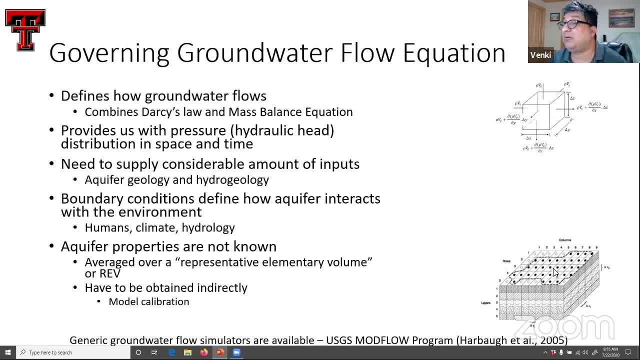 different locations, calculating the direction of the groundwater flow or the volume of groundwater flow becomes easy. And then we typically use a model like this and say, okay, if I put a pump here because somebody wants to pump water, what does it do? And you know. 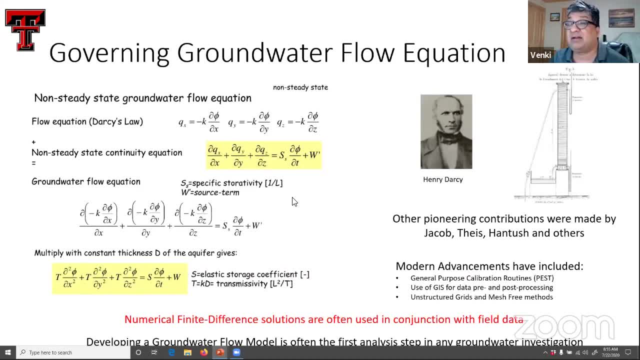 we can calculate those types of things very easily. So again, these are the governing flow water equations. They are partial differential equations. second order: partial differential equations. And t is the transmissivity, v is that hydraulic head and w is the source sink term. 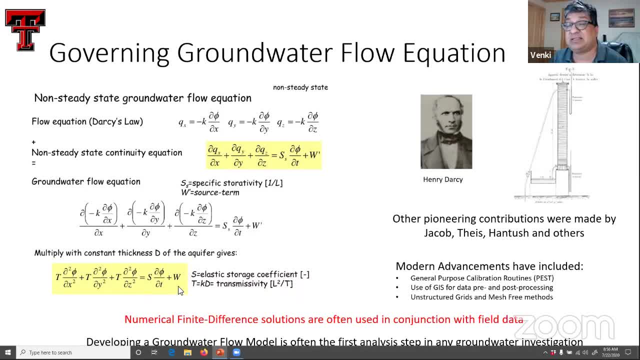 And then s is your storage coefficient And, as you can see, you have x, y, z and t, which are your four states. you know, which are your spatial and temporal coordinates. So what you get is the values in space and time, And this is how this work is done. It all started with this little 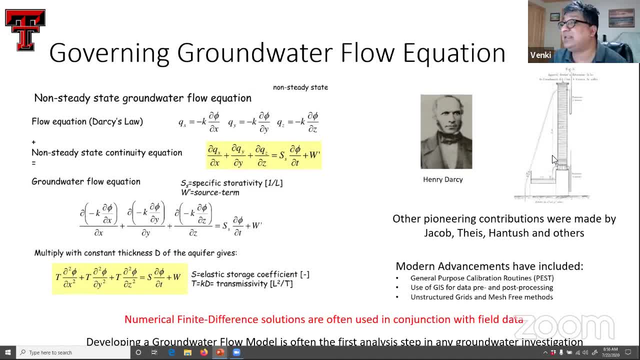 experiment that Henry Darcy did way back in 1857.. Darcy was a French engineer who was tasked with bringing groundwater to the city of Dijon. As you know, Dijon is very famous for mustard growth, So there's a lot of mustard that's produced in Dijon. 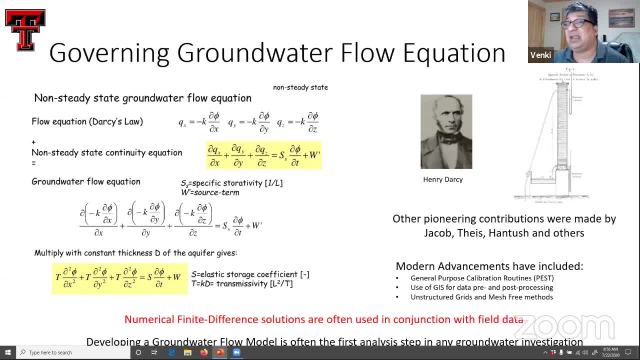 And then. so when Henry Darcy did this experiment, he came out with the Darcy's law, which basically said that the flux of the groundwater is proportional to the head gradient, so that k is the coefficient of permeability or the hydraulic conductivity which depends on the 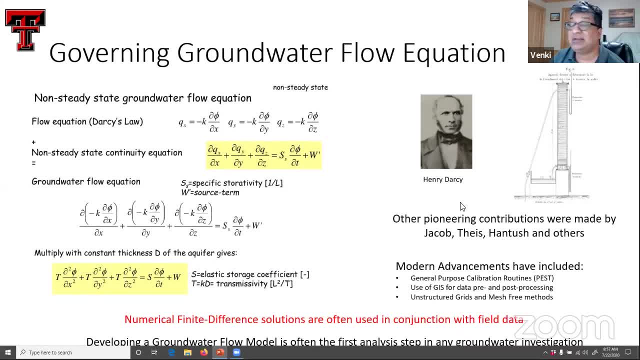 fluid, as well as the geologic properties. Then there was some pioneering contributions made by several other researchers- Jacob Ty Santush- who eventually helped us get the model in this form. More recent advancements have been that we have some general-purpose calibration routines. 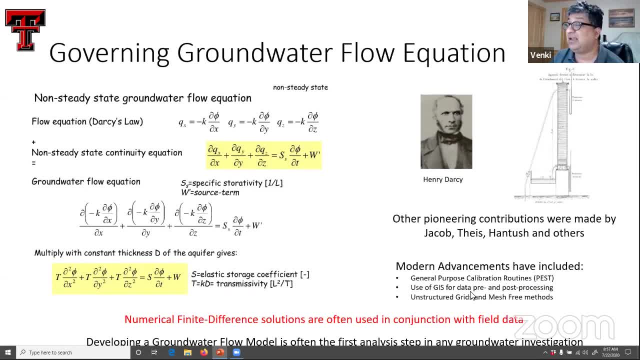 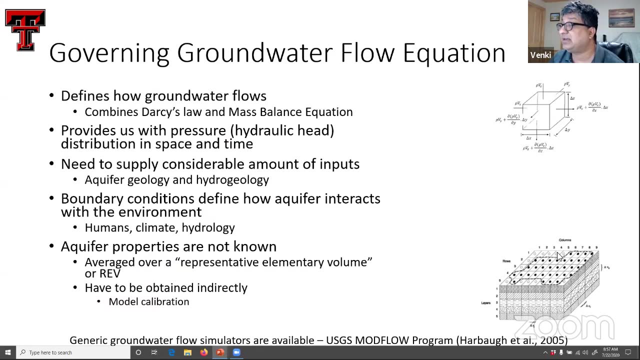 particularly PEST, and then the use of GIS for data pre-processing and post-processing, And there is quite a bit of interest in looking at unstructured dairy grids and mesh-free methods to do faster computations or to not be limited by how we discretize these domains. 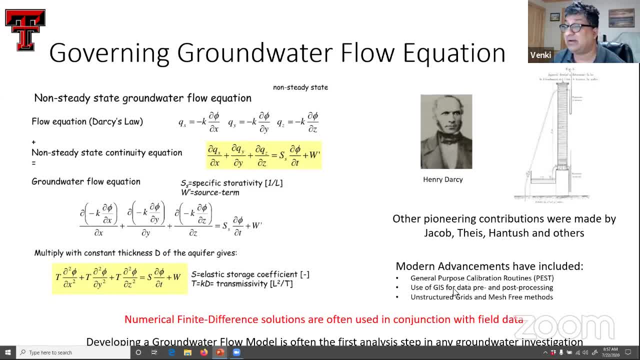 So those are some of the very recent advancements that have happened in this area. So you know I'm very happy to be here, Thank you. So development of a groundwater flow model is the first step of any groundwater investigation. If you're doing a water supply project, your models are going to be very large. 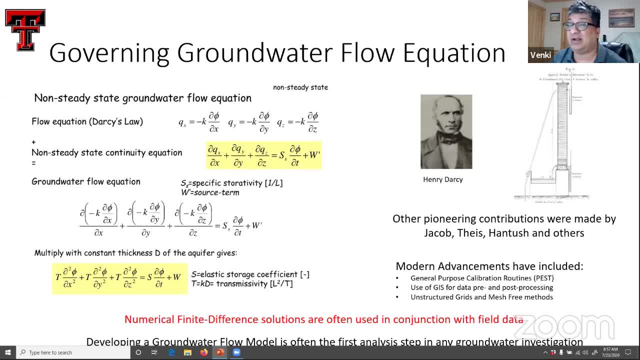 They usually span hundreds of miles, hundreds of kilometers or square kilometers, And when you do a contaminant transport problem your domain is fairly small, typically few square kilometers at best. So the difference really between the two is the scale, But in terms of how those models are set up for the flow, they're essentially the same. 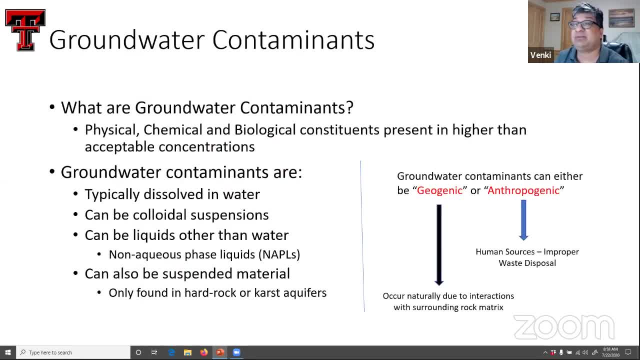 So, coming to the contaminant portion of the things, what are groundwater contaminants? Well, groundwater contaminants are physical, chemical and biological constituents that are present in water in higher than acceptable concentrations. So if you take groundwater from a well, it's going to contain a lot of these constituents. It'll have some dissolved solids in it. 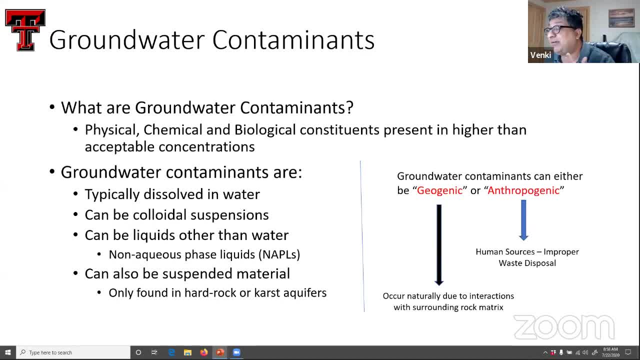 It'll have a whole host of chemicals because that water has been in contact with the rock matrix for millions of years, in some cases tens of thousands of years at the very least. So it has that opportunity to interact with that rock matrix And there's a whole bunch of geochemical reactions. 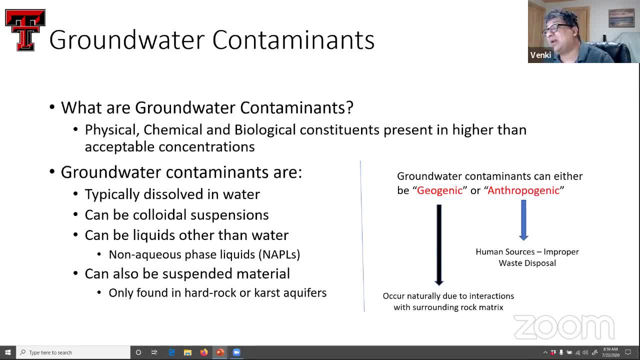 that have taken place and caused contaminants or caused chemicals to dissolve in that water Groundwater systems. the pH typically is around 6.5 to 8.5. In most parts of the world, So that also means that they are very biologically active zones. So 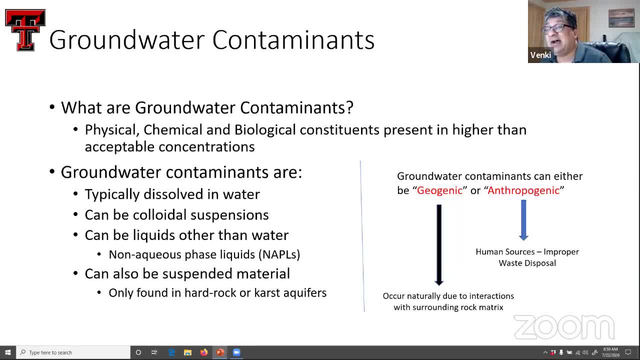 if you have a shallow aquifer, you typically have oxygen, So you will have aerobic bacteria. And if you're going to deeper aquifers where there is not enough oxygen, you will end up having anaerobic bacteria, bacteria that use sulfur, iron or some other. 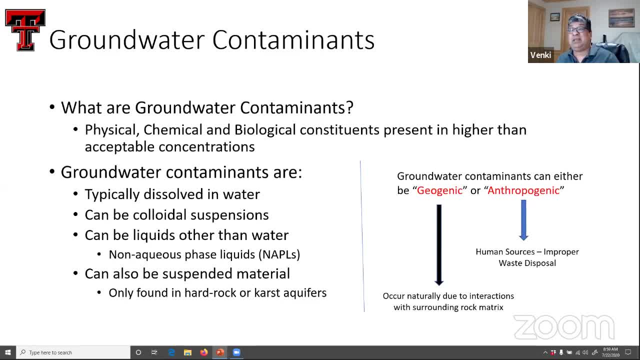 you know even carbon dioxide For breathing, for deriving energy, as we do with oxygen. So, as humans, we breathe oxygen, so we are aerobes. But there are anaerobic environments where there is no oxygen and you still see life forms, but mostly microbial life forms, that are present as well. So just because 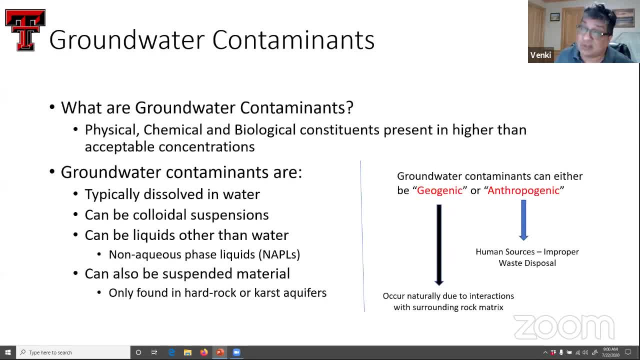 those chemicals are present or those microbes are present doesn't necessarily mean that groundwater is contaminated. Groundwater is contaminated when the levels of these chemicals or these biological constituents or even physical constituents like heat. If you go very deep into deep formations you get geothermal energy, so the water can be very hot And as a result, you can't use it. So 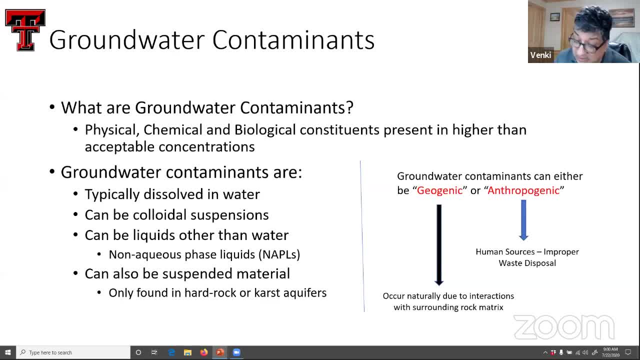 you want to dissipate that heat before the water can be used. A lot of times you may want to exploit that heat to heat up, something sort of like you know, heat up buildings. So people use that to do those types of things as well. But generally speaking, elevated levels have to be. 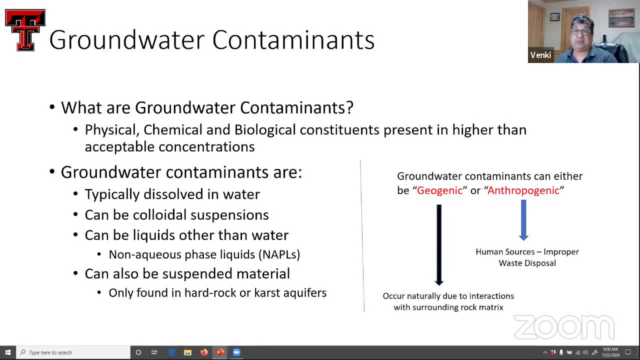 at least before we can use it for our purposes. Groundwater contaminants typically are dissolved in water. because the sand acts as a filter, You could have colloidal suspension. Most of the microbes that you get are actually colloidal suspensions. Milk like milk, you know you. 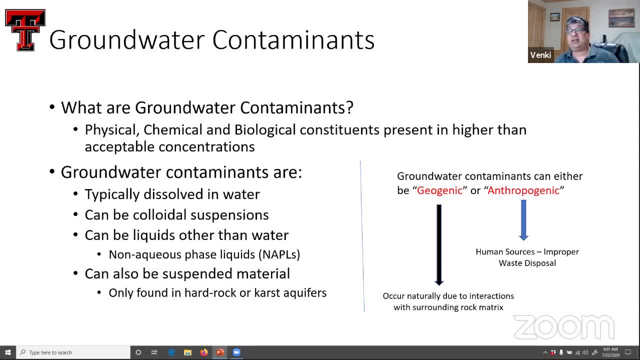 know that that is water and have colloidal suspensions in milk. But generally speaking, you need to do very high filtration, you need to have very high filtration, you need to have very high filtration to separate those two. It's almost like they're mixed. 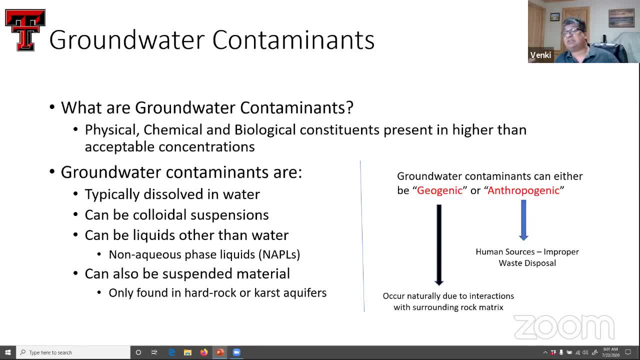 There can be liquids other than water. These are called the non-AEA space liquids, especially if you have petroleum type contaminants or trichloroethylene- a lot of these organics which tend to be hydrophobic or repel water or very sparingly soluble in water. 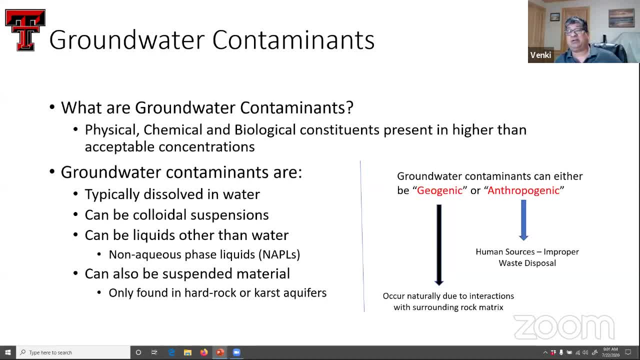 They tend to be present as a separate phase or a separate liquid, and that causes some challenges. And there can also be suspended materials. Typically, you don't see this in sand and gravel formations, but you can find suspended materials in hard rock or in karst aquifers. 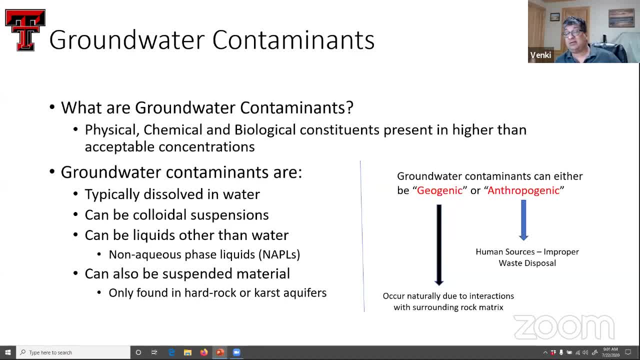 Hard rock aquifers are what's there in most part of South India. These are the deeper bedrock aquifers where you have conduits or channels to which water moves Karst. there are some karst near the Tiputla and Andhra Pradesh, but these are basically. 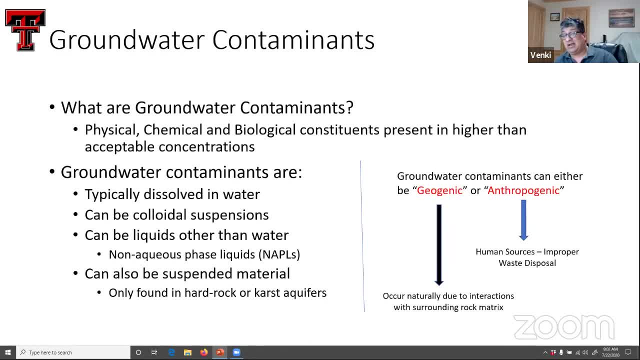 limestone formations, So the water dissolves The limestone and then creates conduits for water flow, So there are karst formations there as well. So when it comes to contaminants, humans do cause contamination of groundwater, So those are called anthropogenic contaminants. 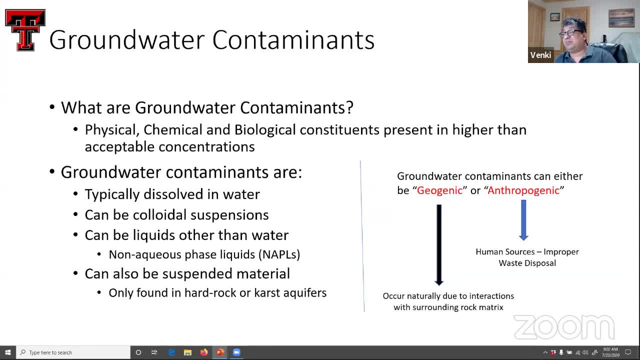 largely because of improper waste disposal practices, But there is a lot of geogenic contamination that occurs. That's because there are chemicals in the rock that get dissolved in water and make the water unfit. We talk about fluoride problems in Andhra. That's largely a geogenic contaminant. 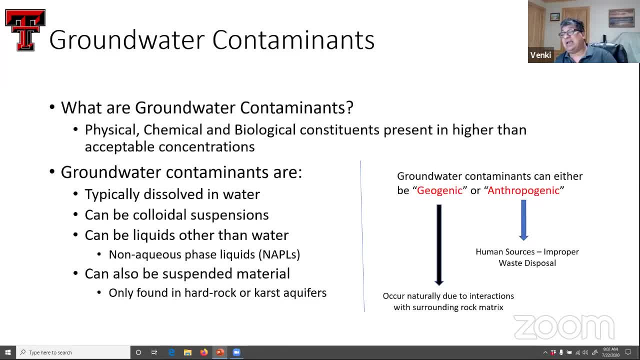 Arsenic and fluoride are two very large geogenic contaminants that we worry quite a bit in India as well as in the US. Like we're in Lubbock and in Texas, where I study and teach, That's a big issue for us as well. 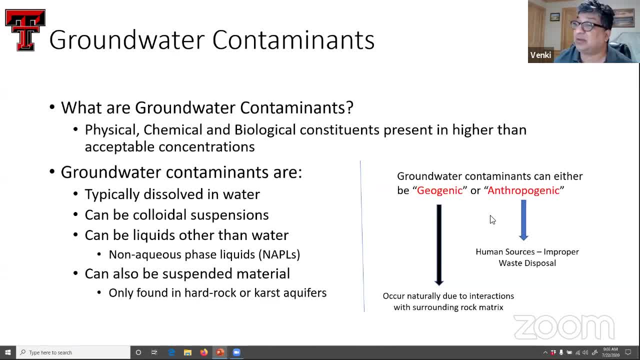 So we have quite a bit of geogenic contamination, but there is also anthropogenic contamination. US has a lot of geogenic contaminants. There's a lot of geogenic contaminants. There's a lot of geogenic contaminants. There's a lot of geogenic contaminants. 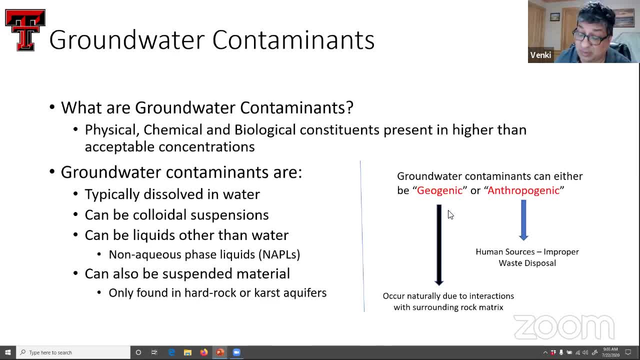 Usually the difference between these two is that the geogenic contamination is spread over a very large area, So we don't actively treat geogenic contamination. What we do is we usually pump the water out and treat the water that we have pumped to reduce the geogenic contamination. 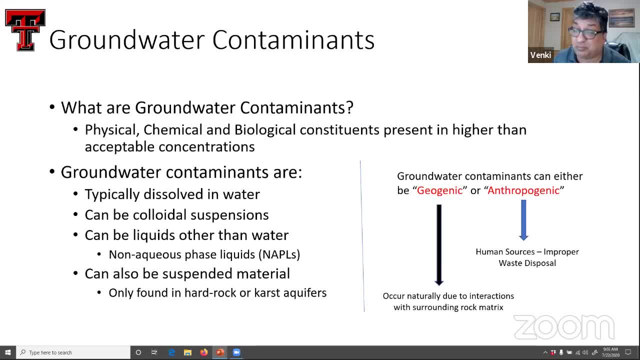 So there is fluoride. Fluoride has the matrix maybe that it may extend over hundreds of square miles, sort of like hundreds of square kilometers. So we really cannot actively, We don't want to mediate this geogenic contamination zone. 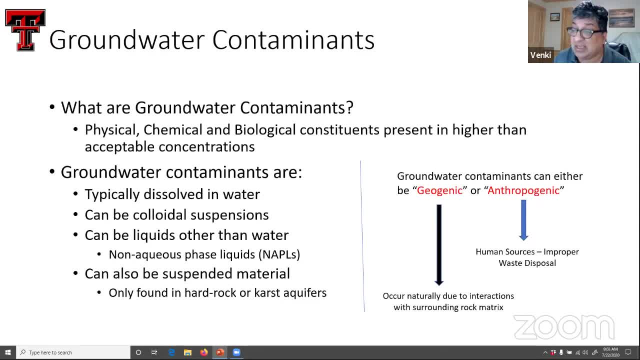 What we do instead is we pump water and before we supply it to people for municipal water supply, we remove that fluoride or bring it down to a certain level. So that's the strategy that we use When it comes to anthropogenic contamination. 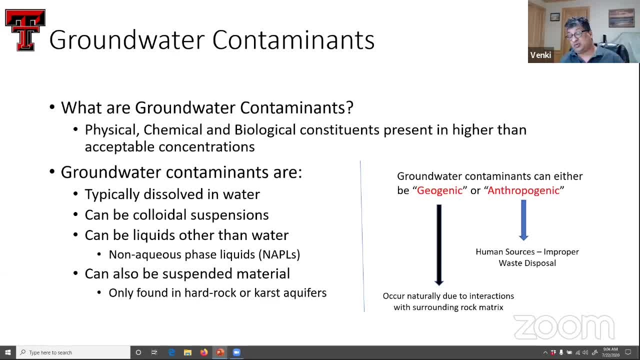 this is usually: there is a leaking tank or some other source that is much more localized, And then we actively treat that groundwater to remove those trace chemicals and deal with it. So the source is very large, We just pump water and treat it as necessary. 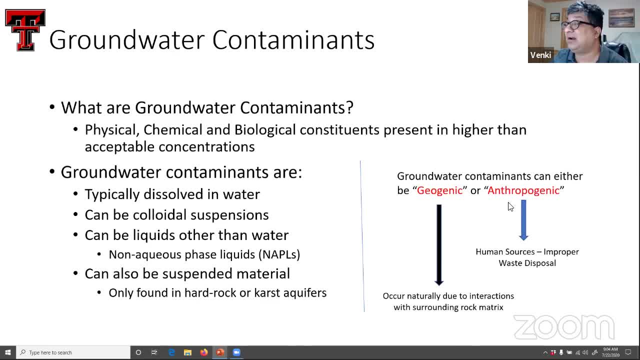 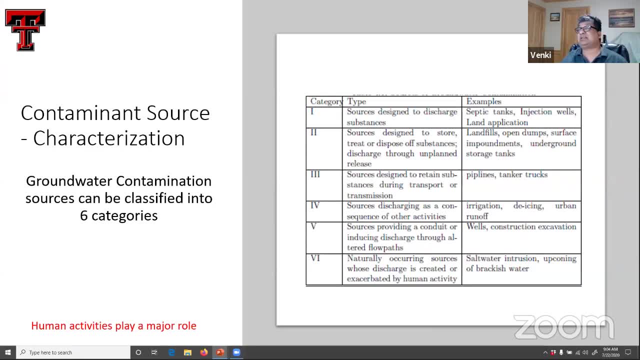 If the source is small, we tend to treat the groundwater and get rid of that source as possible. So we can classify the sources in six different ways. We have sources that are designed to discharge substances- septic tanks, for example, injection wells. 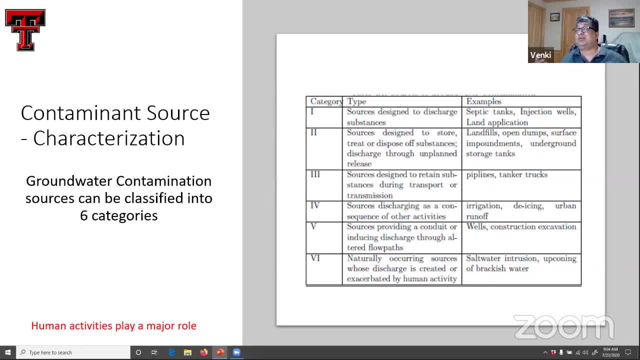 Sometimes we do land application of waste because we use them as manure. The sources used to dispose substances: these are the sources that are designed to dispose substances. These are the sources that are designed to dispose substances. These are the sources that are designed to dispose substances. 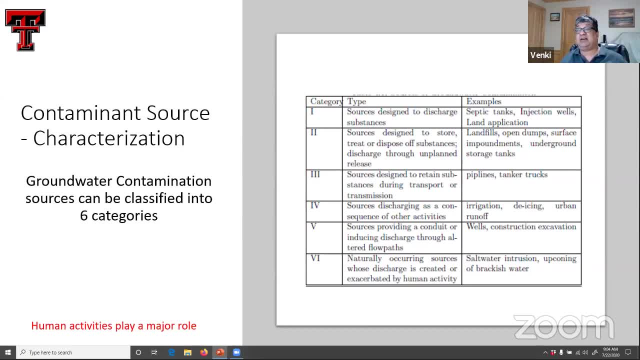 These are your landfills, these are your impoundments, These are there are sources where you take substances to transport, like pipers, pipelines, tanker trucks, And then there is consequence of other activities. So when you do irrigation for farming, 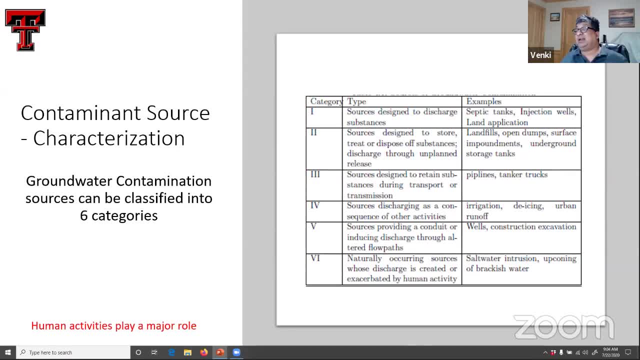 you put fertilizers, you put pesticides. You're not really trying to contaminate your groundwater, but some of that excess can leach off and eventually get into groundwater systems Sources. there might be a source and you may create a conduit by constructing a well. 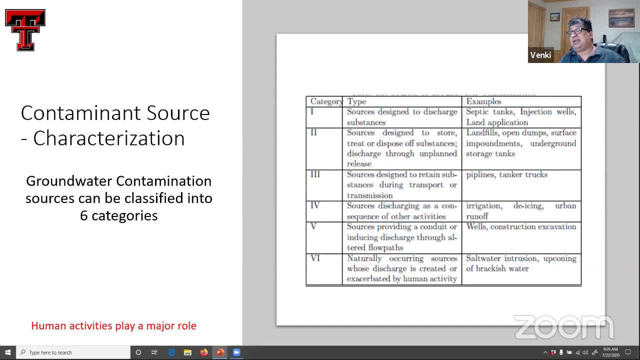 or doing some excavations. So again you have to get permits when you put wells and do the excavations to ensure that you're not contaminating the subsurface accidentally as part of your construction activities. And then there are some naturally occurring sources that get exacerbated by human activity. 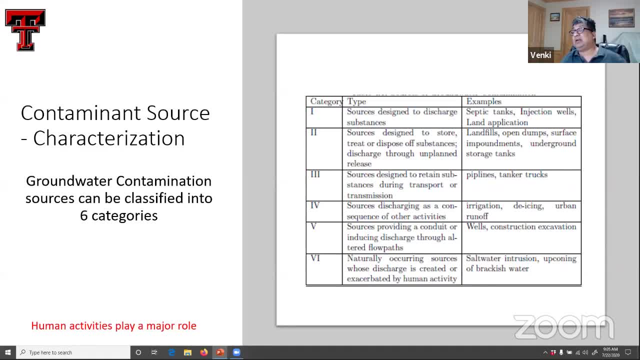 Things like saltwater intrusion, particularly important in coastal areas. upcoating of brackish water. There's quite a bit of brackish water in the deeper formations of the earth And if you're not careful with pumping, that water will actually actually. 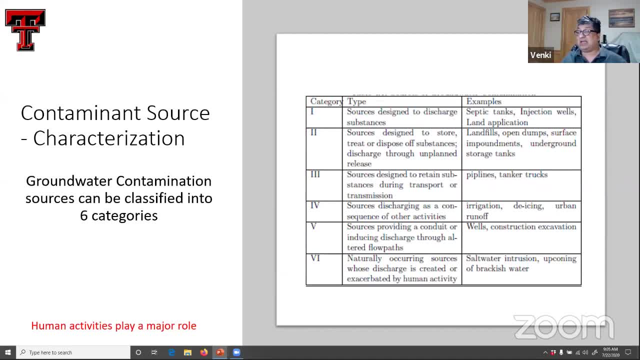 actually come into the shallower portion, So there is unstable water flow. that happens because of density differences And that phenomenon is called upcoating. So human activities, as you can see, play a major role, Even though the sources are natural. 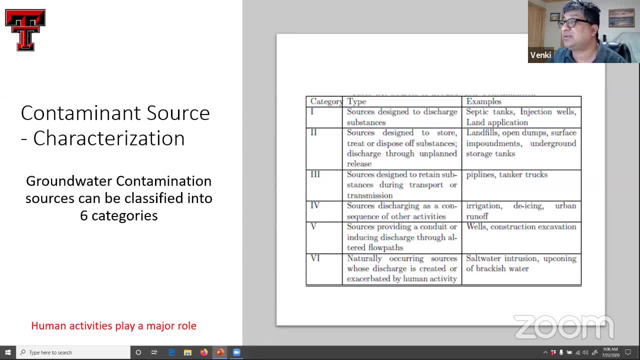 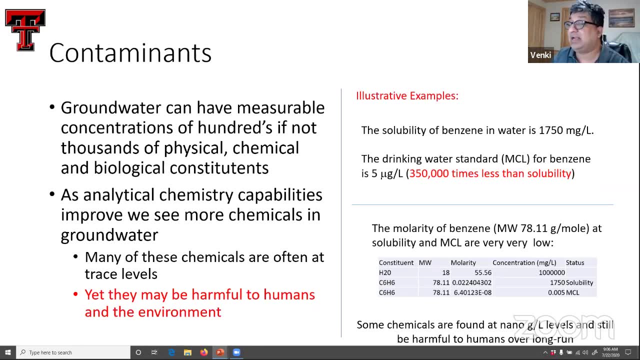 a lot of times humans exacerbate those sources. So the issue with groundwater a lot of times is that water is the dominant chemical in groundwater. So if I take a typical groundwater system, the molarity of water is about 55.56 moles per liter. 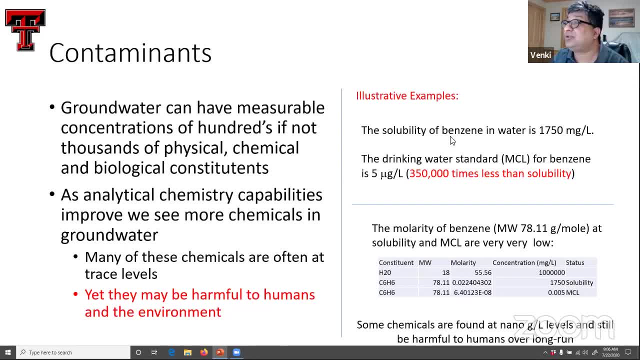 So that dominates. And as an example, I'll show you benzene. Benzene is something you will find in petrol, So it's a big component of petrol. It's carcinogenic, It causes cancer. It's one of the few chemicals 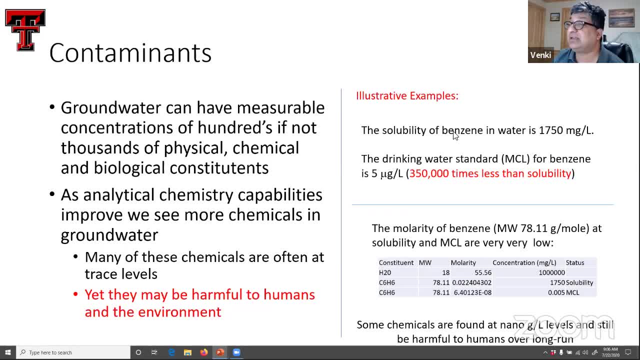 that have been proved to cause cancer And I've just. I think we causes cancer, but we know it causes cancer. The solubility is about 75 milligrams per liter. What does it mean? in terms of moles At solubility, molarity is only about 0.02.. 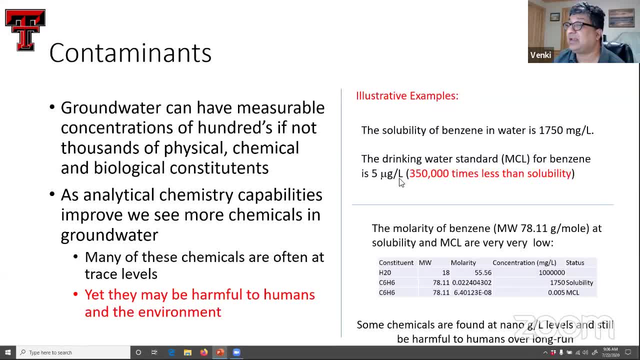 But the drinking water standard for benzene is five micrograms per liter. This is milligrams, This is micrograms, So it is about 350,000 times. So 350,000 times less than the solubility. So even very, very small amounts of these chemicals. 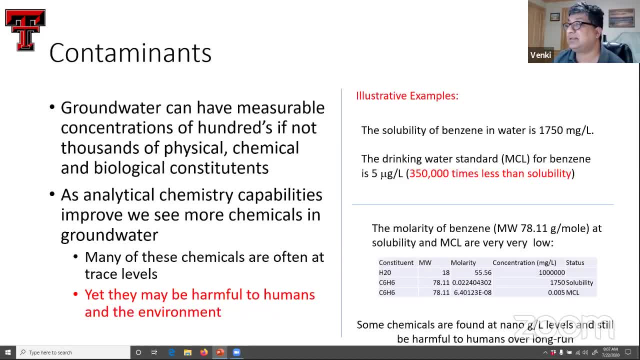 can post toxicity to humans, And that's what makes groundwater remediation, of groundwater transport very challenging, because we have chemicals at very, very, very low dilutions, especially if I want to bring it to drinking. So if I have it at solubility it's about 0.02 moles. 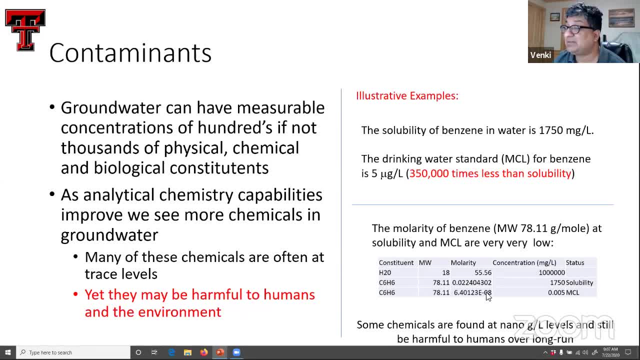 If I want to bring it at the drinking water standards, it's about 6.4 times 10 to the negative eight moles Okay. So it's almost like 0.6 milligrams per liter. It's nanomoles. 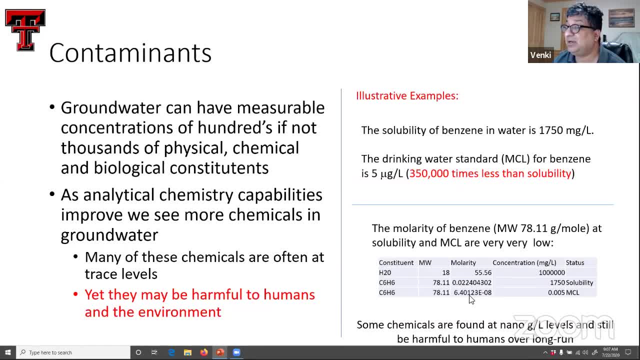 So we are going from like two millimoles at solubility to about a nanomole. So that is a huge, you know several orders of magnitude of cleanup that we have to do to meet our drinking water standards. So that's one of the challenges. 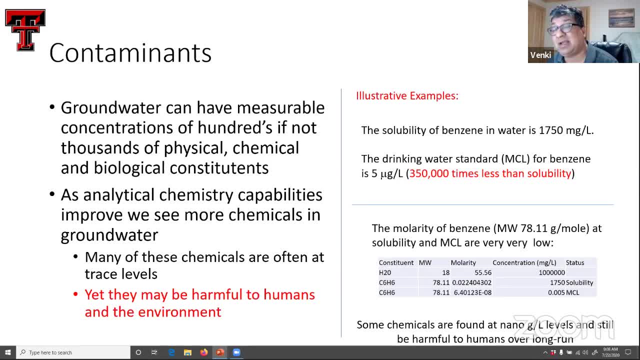 And as our analytical chemistry capabilities have become better and better over the years, we are able to detect more chemicals. So when we detect more chemicals, naturally there is a concern that what are these chemicals going to do to us when we get exposed to them? 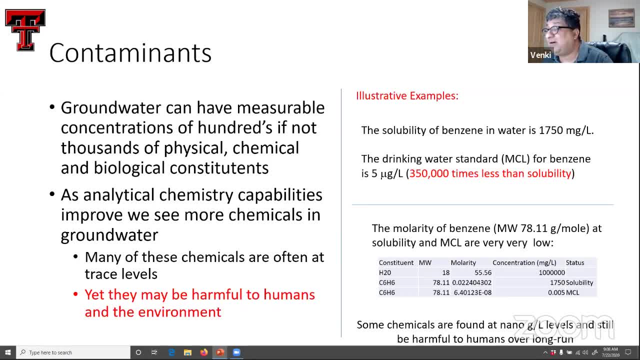 Some of the new chemicals that we are looking at are pharmaceutical products, for example. So people take a lot of medication and then you know it gets flushed down. They pass that through the urine or crecia. eventually it gets into the subsurface environment. 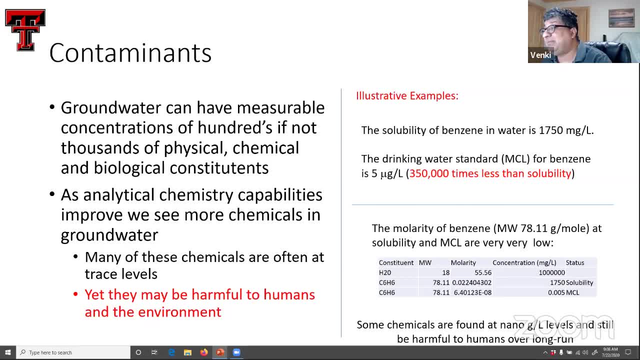 It can get into the water and somebody else who doesn't need that chemical might be getting very low doses of it through groundwater ingestion. So what is the risk? Are they getting affected by something that they shouldn't be getting affected? So some chemicals are found at nanogram levels. 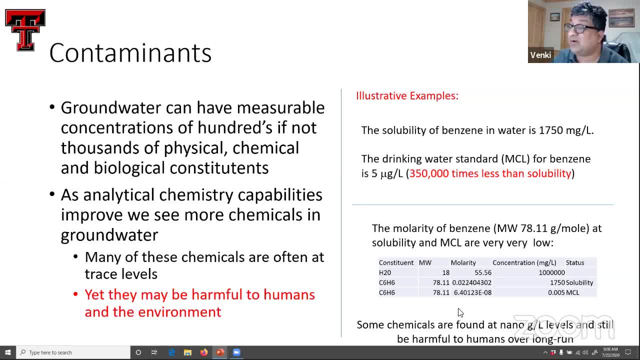 and they still can be harmful to humans over the long run. So a big challenge when we deal with groundwater contamination is dealing with very, very, very low concentrations or trying to bring that water or the chemicals in that water just to you know, to us. 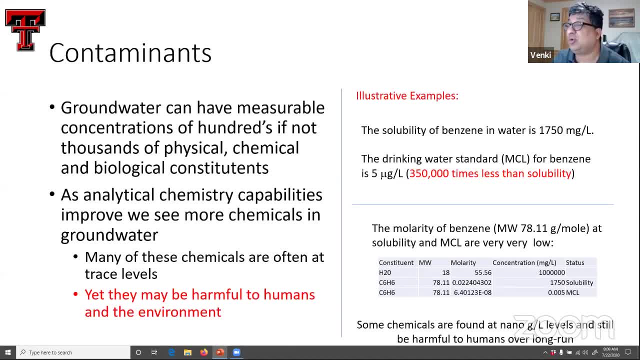 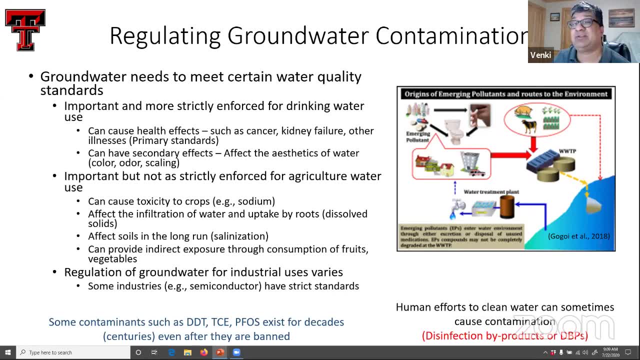 So that's a big challenge for us. We have such low concentrations that it's virtually undetectable. So that's what the groundwater quality is about. That's what groundwater regulations are about. Typically, we put what is known as some health effects. 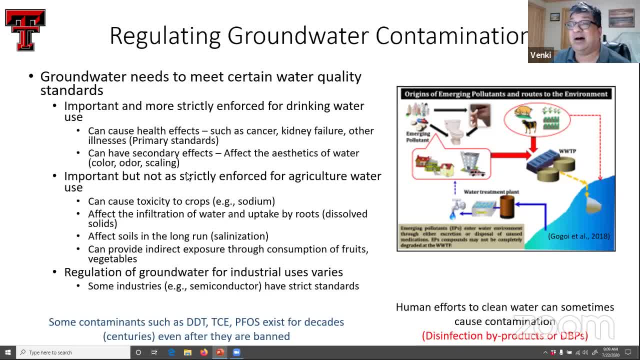 which or there are some secondary effects And in some places we don't strictly enforce it, especially for agricultural water use. But they can also be important, because when you consume fruit and vegetables that are grown with contaminated groundwater, some of the contaminants can actually get accumulated. 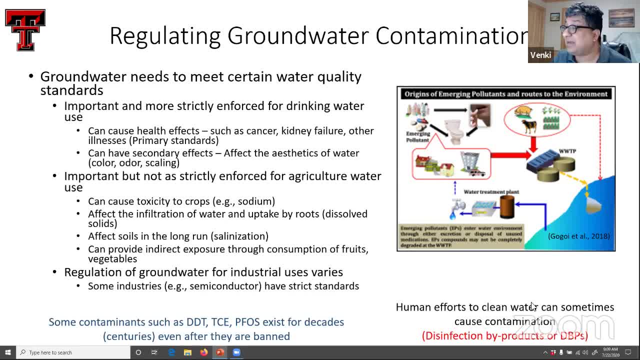 in fruits and vegetables and cause indirect pathways. Sometimes we want to clean water So we put like chlorine and disinfectants, and those disinfections can actually cause harmful byproducts that can be problematic to us as well. And then there are some contaminants like DDT. 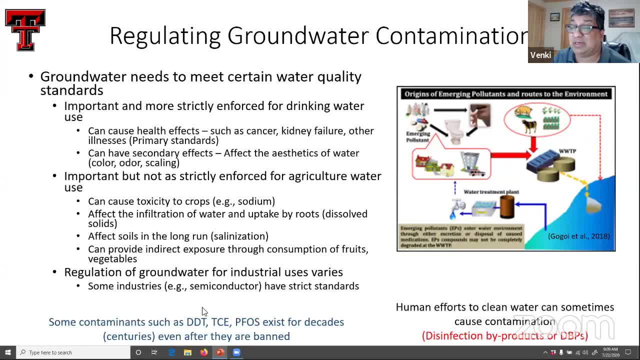 DDT has been banned for a very long period of time, but we can still detect that in groundwater systems, PFAS or perfluoroalkyl substances. we've got very long chain. We've got a very long chain of perfluoroalkyls. 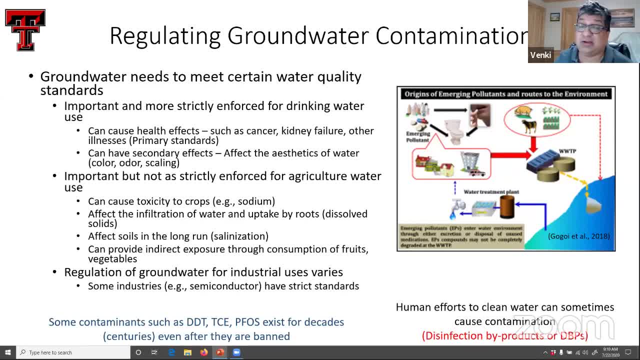 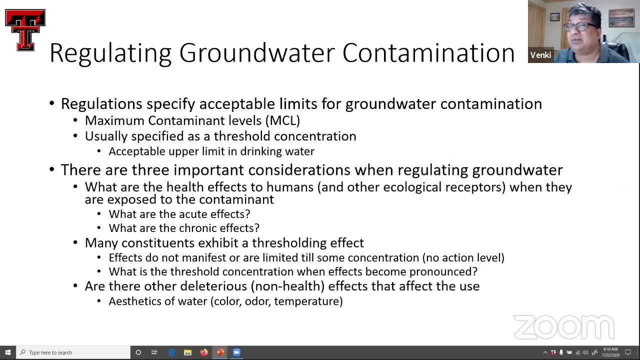 They are the hot topic now in groundwater. They're ubiquitous, You can find them in many locations, So those are of interest as well. So the groundwater contamination is regulatory. There are regulatory drivers And what we want to do is how do we get these regulatory drivers? 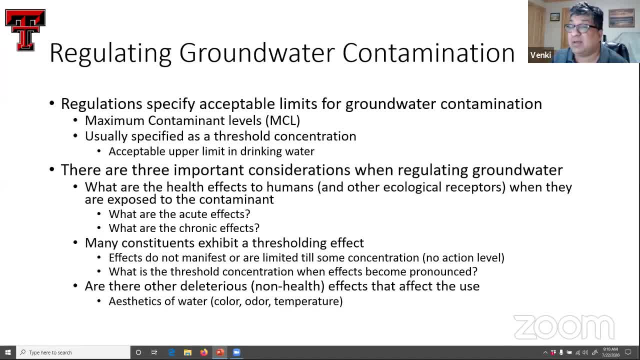 We get them based on what risks do they pose to humans? Typically, there is a level below which they will not pose risks, And then there is a level below which they will not pose risks, And then there is a level below which they will not pose risks. 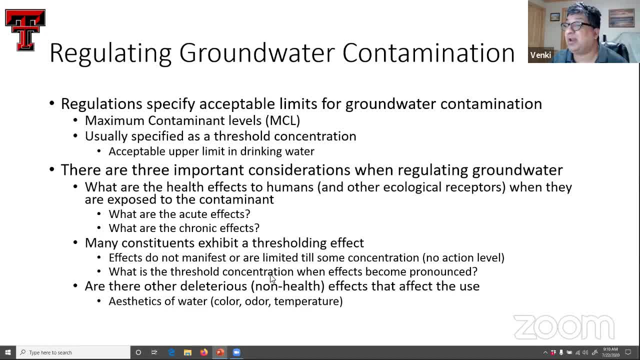 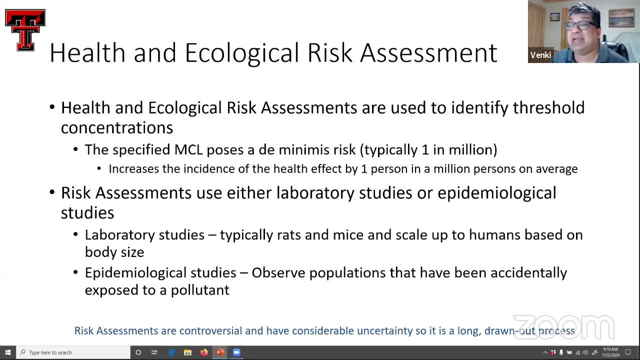 And then there is a level above which they will not pose risks. So that threshold is what we want to clean up to, or that's the new action level. So we do what are called as health and ecological risk assessments to identify those threshold concentrations. 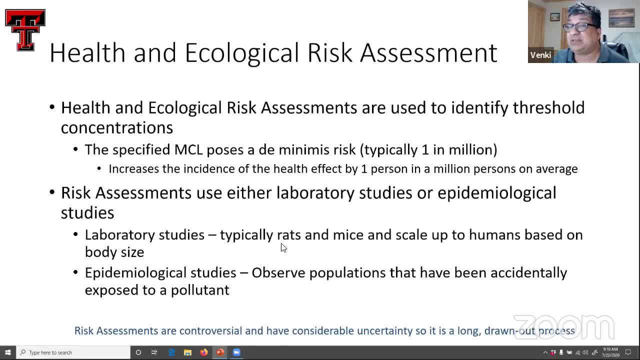 Again, these tend to be really controversial a lot of times because we can't expose humans intentionally to this chemical, So we expose them to rats or to mice and then try to scale up to humans. So how good is the metabolism in dry mats or rice? 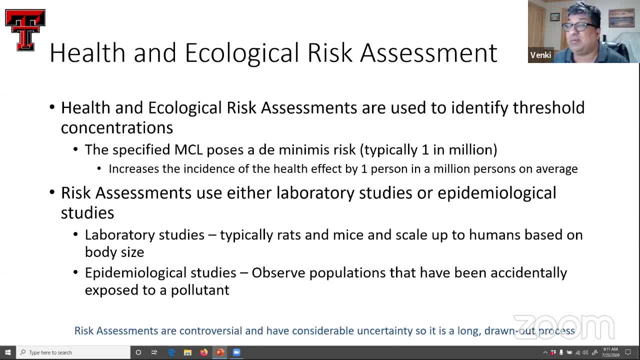 rice compared to the metabolism of humans. there's a lot of debate that toxicologists get into, Or we use epidemiological studies where we observe populations that have been accidentally exposed to a pollutant and see what has happened to them, And again, of course, this is also a very 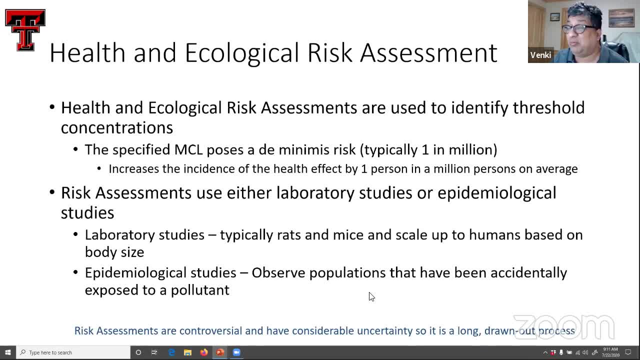 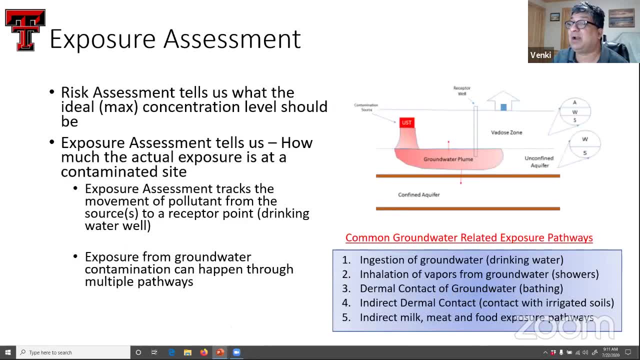 challenging field. but once we have a standard it goes through a long process and then they do have a considerable uncertainty associated with them. but we try to regulate to that level. That is the risk assessment part. The exposure assessment part tells us what is the current level of risk or how much is the exposure. So typically we have a contaminated. 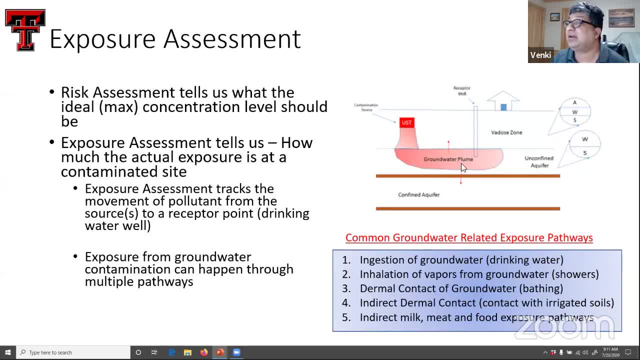 site Contaminated, leaching creates what's known as a groundwater plume. The plume is basically where the groundwater is contaminated And if you have a well, we start pumping that water and we start taking that groundwater So we can ingest that groundwater as drinking water. We can. 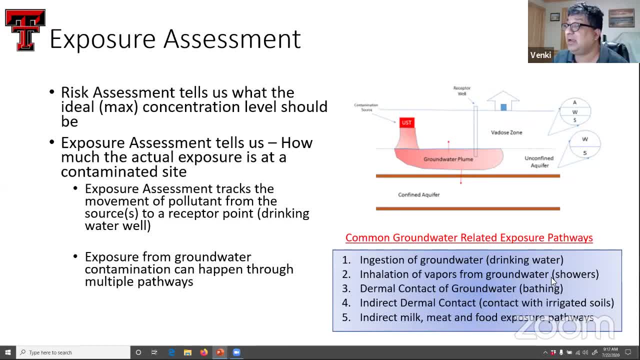 ingest that groundwater as drinking water. We can ingest that groundwater as drinking water. We can inhale vapors, especially if you're taking showers- very hot water. We can come into dermal contact during bathing. We can also come into some indirect dermal contact by irrigating. 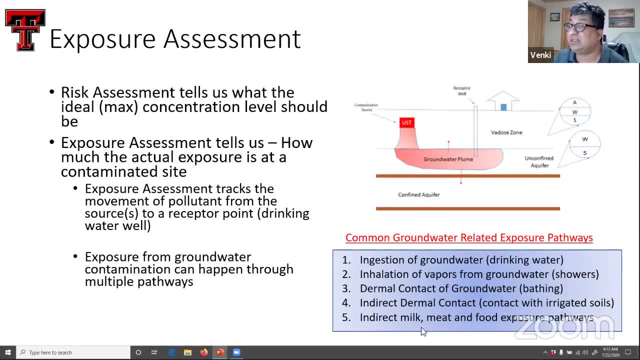 the soils around it and then getting exposed to that soils or indirectly through milk, meat and food exposure pathways. We might use groundwater to produce meat, food or milk and get exposed that way. So there are many ways in which groundwater actually affects and not just in 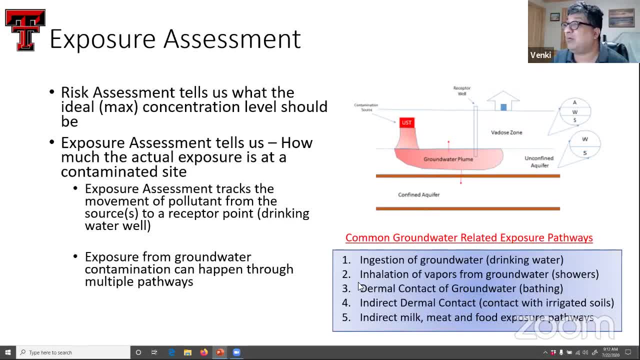 terms of your drinking water, but also in terms of how much water is ingested into your body. So there are many ways in which groundwater actually affects, and not just in terms of your drinking water, But there are other pathways to which groundwater contamination can happen, with humans as well. So the exposure assessment is the 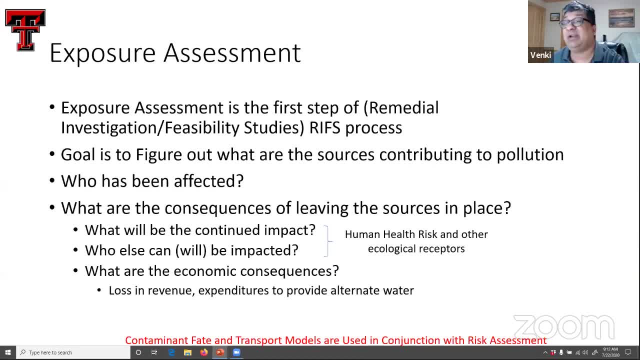 third step of what you would call the RFS process, the Familial Investigational Feasibility Study process. The goal here is to figure out what are the sources contributing to the pollution. who is being affected? And the first question we ask is: 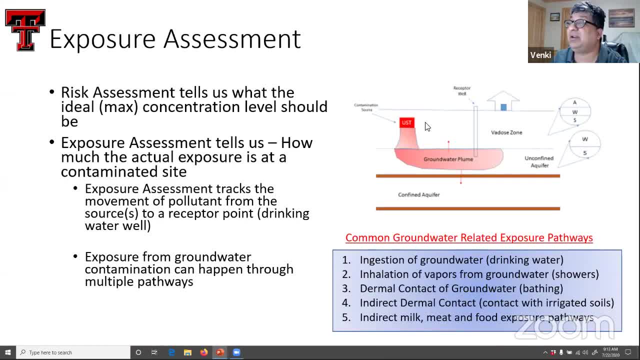 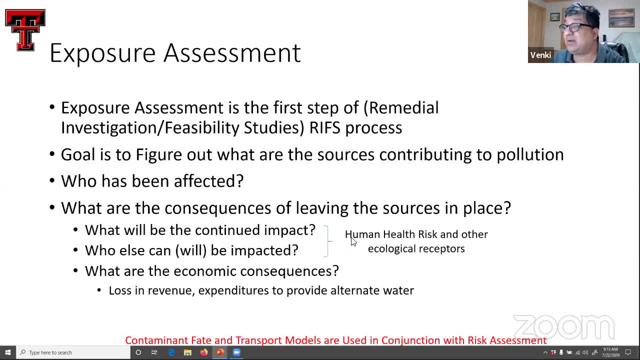 what happens if I leave that source in place, If I were to leave this contaminated soil or this contaminated groundwater in place, what is the impact? What is the risk to humans And what is the risk to other ecological receptors? And then what are the economic consequences? What's the 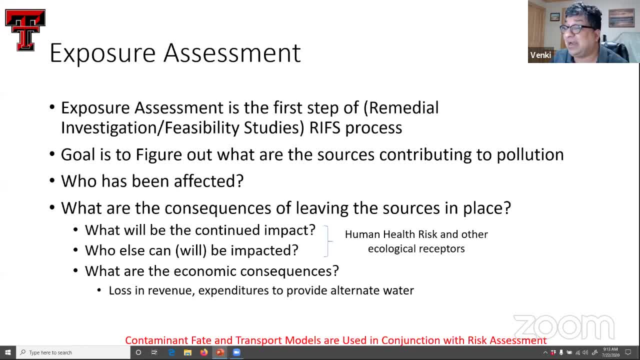 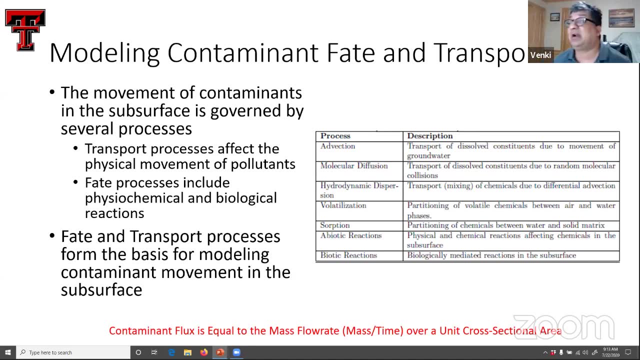 loss of revenue? What are the expenditures involved in losing that water or providing alternative source of water? What do we do with that? So those are some of the questions. So we use contaminant freight and transport models. Freight and transport models are a lot more complicated than your groundwater flow models. 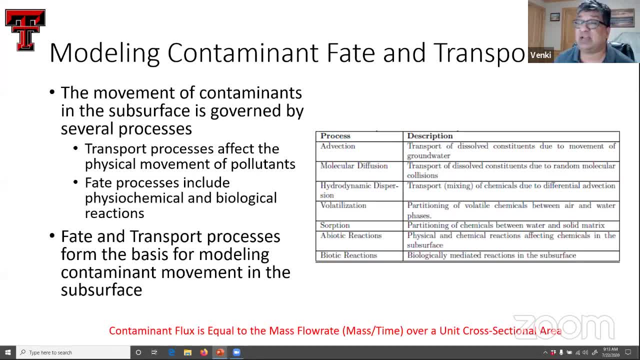 because the contaminant movement is affected by many processes, not just the flow of groundwater. So advection is the movement of contamination to the movement of groundwater, which you can have molecular diffusion, You could have mixing, which is called hydrodynamic dispersion. 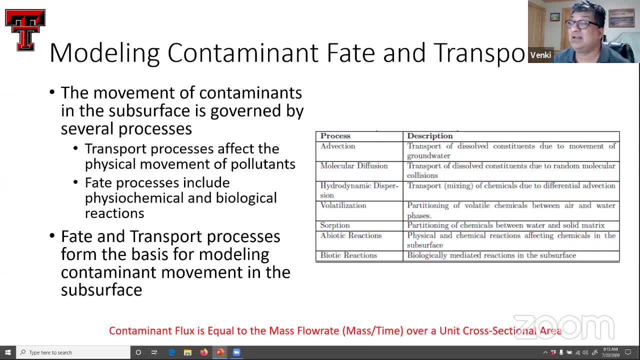 You could for some chemicals to volatilize so they actually get into the air phase. So that might be of interest. Sorption is when we have a contaminant in groundwater partitioning into the solid matrix or the solid matrix. 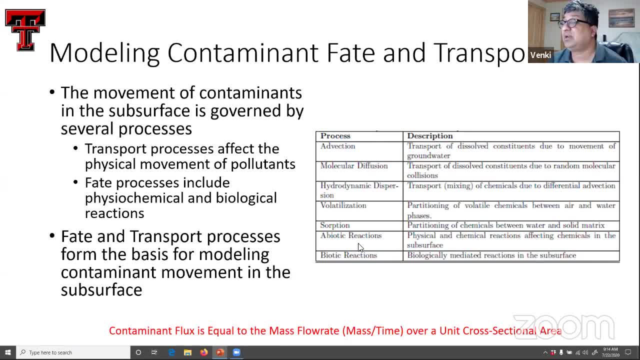 Contaminant getting into groundwater that processes sorption. We could have some physical and chemical reactions happening in the subsurface and biotic reactions that are biological or microbial reactions that are happening in the subsurface. So we have to calculate the fluxes or the mass of change of mass per time associated with each of these processes and put together 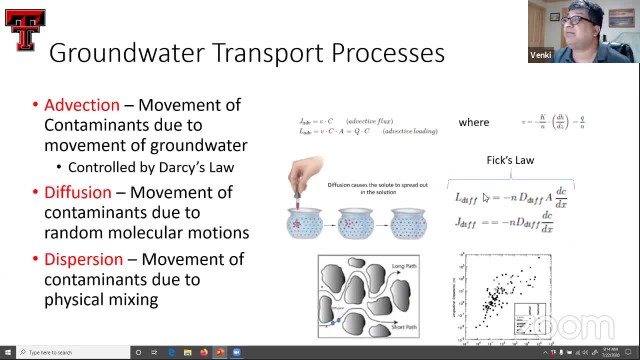 And we use again similar to Darcy's law. we make use of Fitt's law, we make use of Darcy's law to get advection, diffusion, dispersion Parameters. these are what are called transport processes. And then we use fate processes. 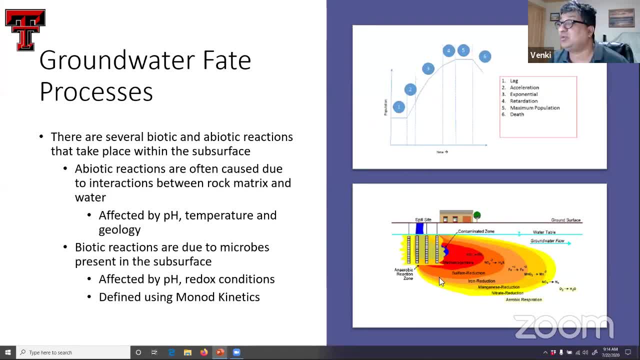 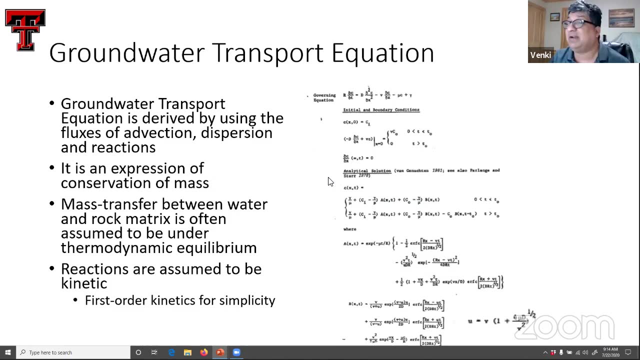 which are basically chemical kinetic processes. So this is very similar to what people do in chemical engineering when they design reactors. So we use those conditions and then put it all together to form equations like this. This is what's called the groundwater transport equation or the advection dispersion equation, And then we can solve them either analytically or numerically. 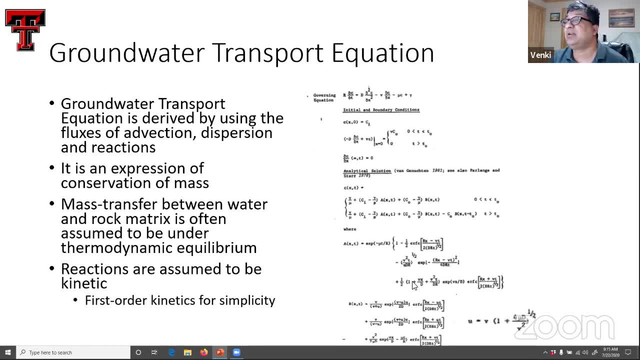 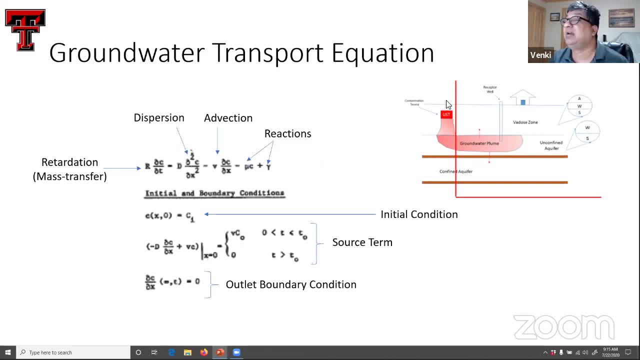 to calculate the concentrations over time. And so here I show you a simple one-dimensional advection dispersion reaction. where there is a source, the groundwater is getting contaminated, and we are tracking that contaminant as it moves through our aquifer system. So as it moves. 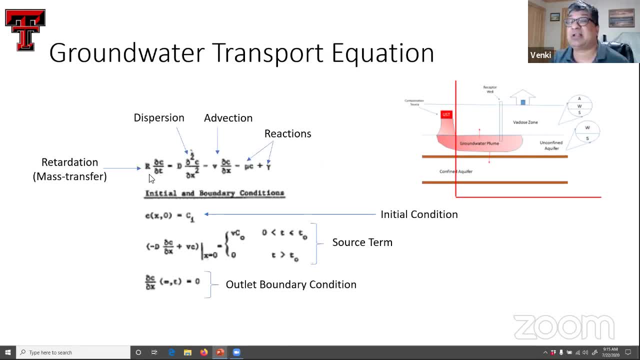 it is interacting with the rock matrix, so that is when there is mass transfer between rocks and the water. So that's the retardation term. There is dispersion, There is mixing going on because it's taking a tortuous pathway. It is not a straight. 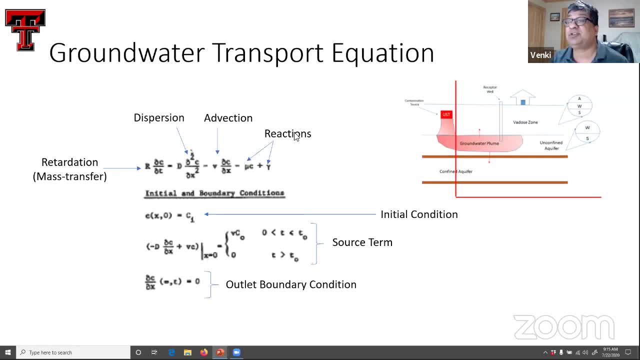 pipe. It's moving through pores, so it mixes, So that's the dispersion, And of course there is a gradient that is causing the groundwater to move in some direction, and that is the advection part. And as all these things are happening, there could be reactions taking place as well, both. 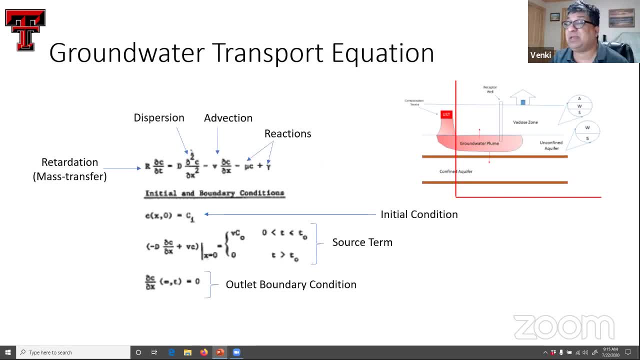 due to microbes and due to natural conditions such as pH changes, rock matrix changes and so on and so forth. So we capture all of these using these models, specify any initial or background concentrations and then we say: what does this source look like? Our first step is to say this: 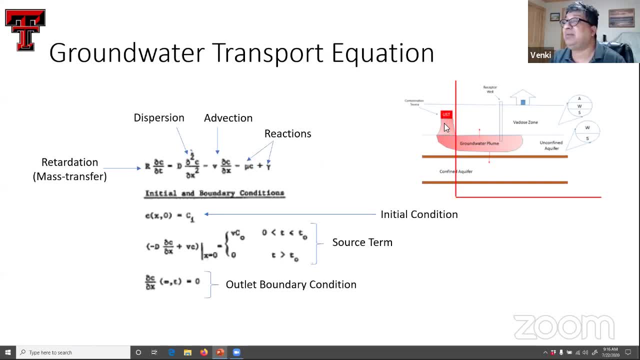 source exists forever and see what the risk is. And then, when we come to remediation, we say: what if we cut down this source by half? What if we remove this? What can we do to do this? But we use a very similar model to figure out what will be the concentrations of this. well, where humans 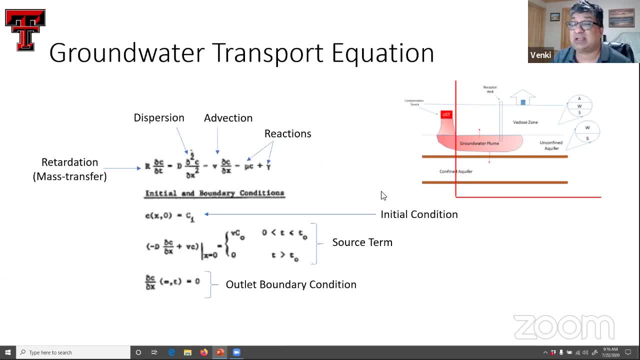 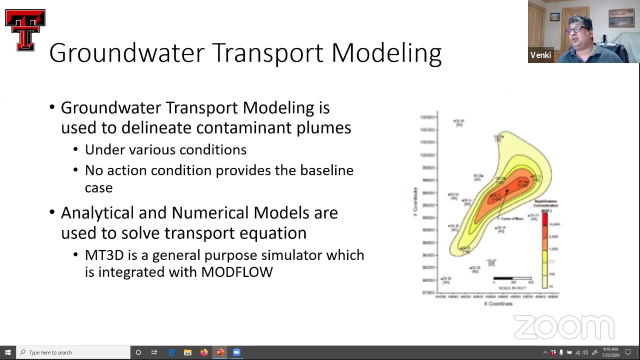 are getting exposed Or some ecological receptor is getting exposed. A lot of times when you go into the two- and three-dimensional models you don't have analytical solutions so you have to do numerical solutions And solving that model numerically poses its own challenges because a lot of those 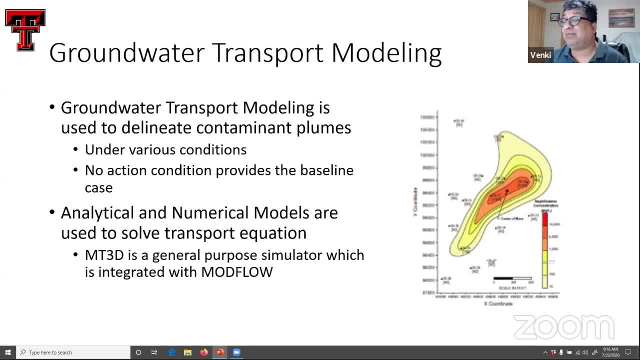 parameters are unknown, So we have to estimate them again by doing field studies and then making some good approximations. So eventually, what we do is we delineate what's for the first place. So we have to find the first place. What's the first place of the plume? The plume is: 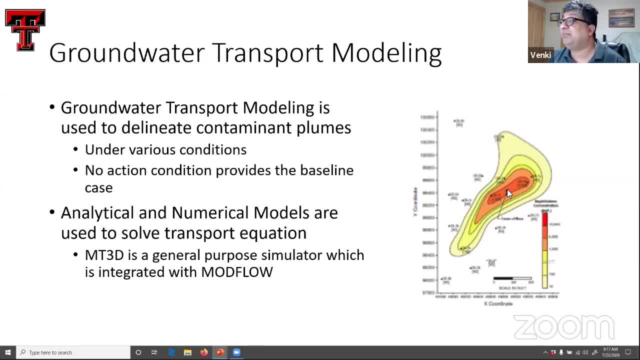 the footprint of that contamination based on some regular limit. The outer limit of that plume is based on some regulatory limit. Of course, the middle of the plume is where most of the contamination is. So we have two things that we want to do. The first thing we want to do is we 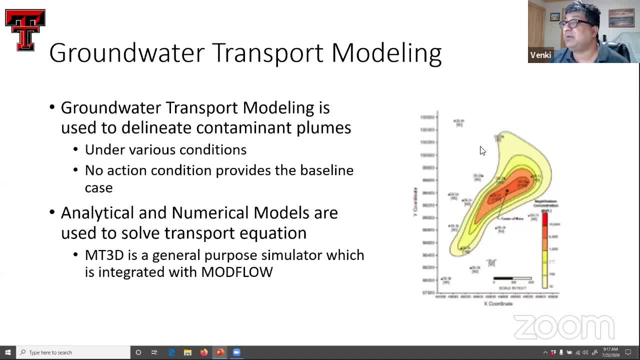 want to make sure this plume stays where it is, It doesn't move forward, Because if it moves forward then somebody else is going to get contaminated. So that's one issue. So we have to control this, shrink this plume or reduce this plume so that the groundwater here can be used as well. 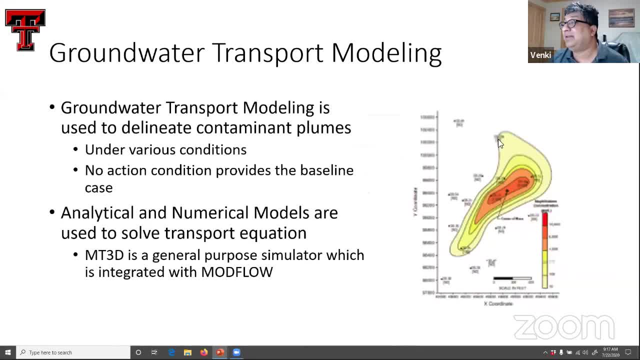 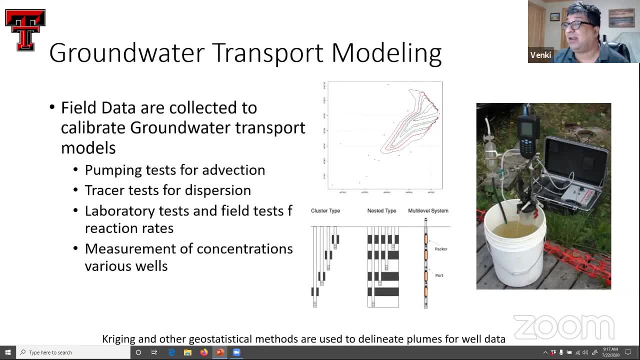 So plume control and then plume mitigation are the two parts that are part of the remediation that we do. We collect a lot of different types of data and we put cluster-type wells, we put nested wells. sometimes we throw in pappers and then sample at different levels. 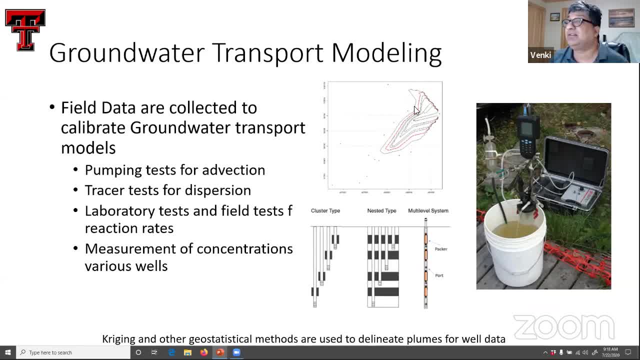 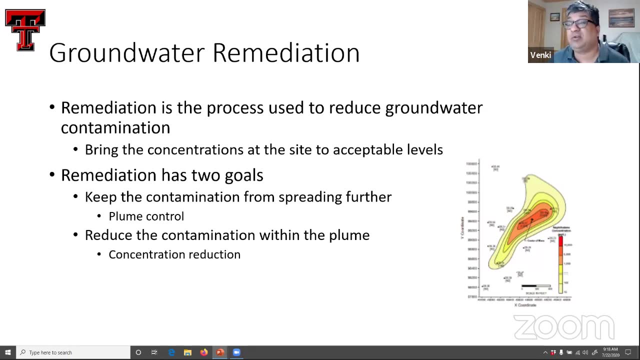 And then we delineate from different wells what the plume looks like, and we make use of a lot of geostatistical methods to delineate these plumes as well. So, in addition to knowing how to solve differential equations, you should also know how to do GIS. you should know how to do. 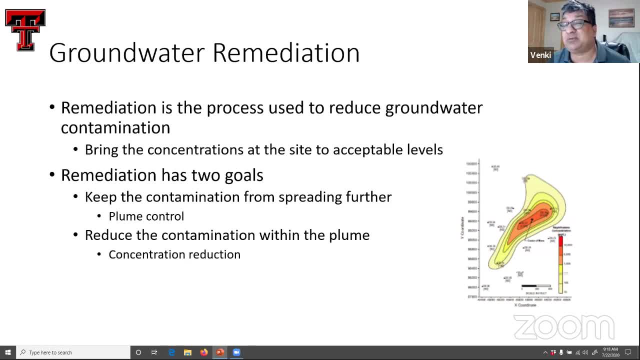 geostatistics. so we use those techniques quite a bit as well to do things And, as I said, the two issues are one: regulate your plume and then reduce your concentration, so that we have taken some of that information and rubbed it in and we are doing that as well. 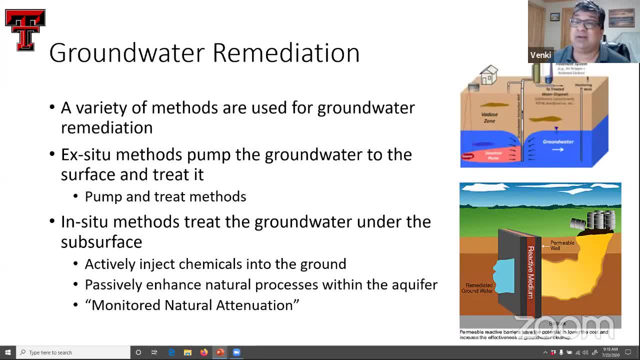 what remediation does. That's the two goals of the remediation. How do we do remediation? Well, the traditional method is what's called the pump and treat, where we pump water and treat it outside. That's our first way of doing it. If you have geogenic contaminants which span over very 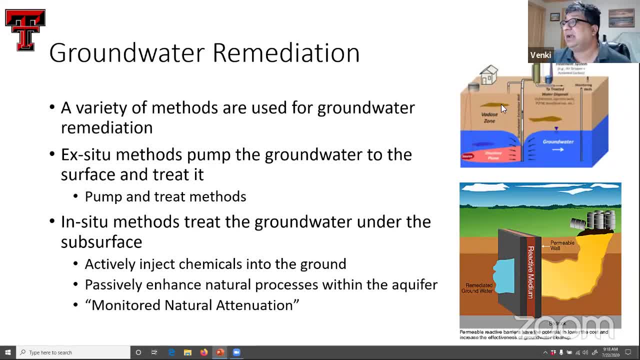 large areas. this is the preferred approach. But what happens is this is a very inefficient process to remove contamination or large-scale contamination, So we have to keep pumping and treating forever to clean up these sites. So if you have an anthropogenic contamination, 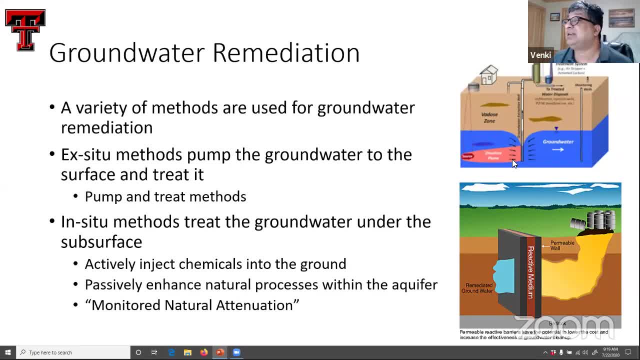 usually we still do this, but we don't do this as much as we used to do in the past. Now we do more passive methods. One passive method is we actually go and put a reactive medium, So we create a trench and then fill it with reactive medium. 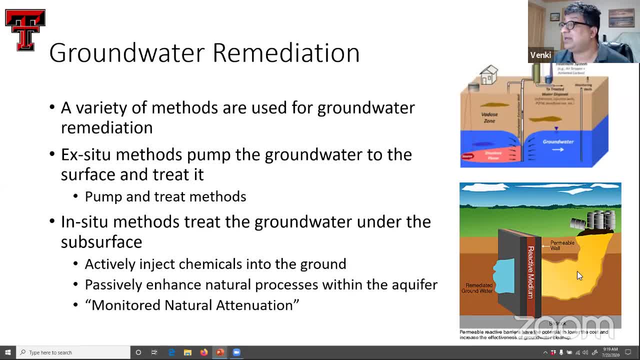 and then make it a permeable vapor, So the contamination actually comes, gets into this reactive medium, reacts and then what comes outside of that is clean water or remediated water or cleaned up water. So this is one of the passive remediation technologies. 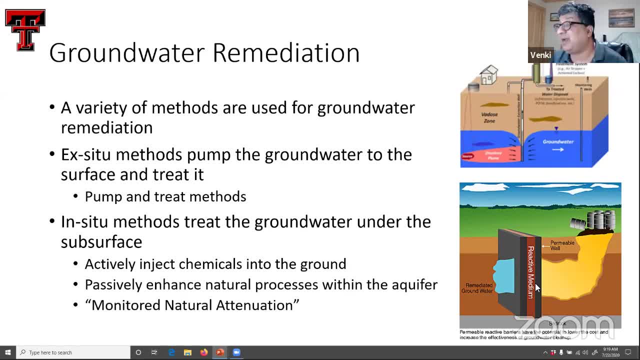 So for this we have to do some sheet filing, We have to do some geotechnical work to create that trench, make sure it's stable, refill it, And then sometimes those pores may clog so we may have to go in periodically back, flush it, remove it or do other things as well. 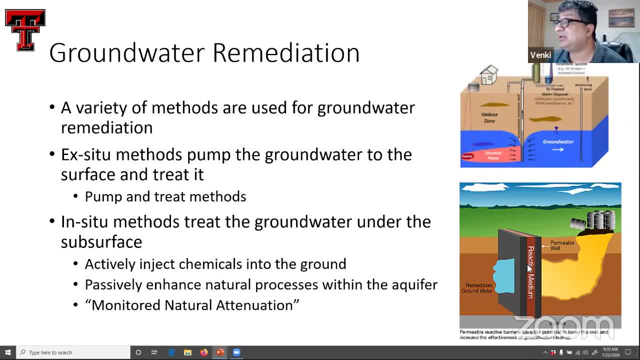 The other option is, if our plume is fairly small, instead of putting a big trench and then putting reactive mediums, we can actually put several wells and then do some passive treatment: put chemicals into the well and treat it in situ. So that's also called in situ treatment. 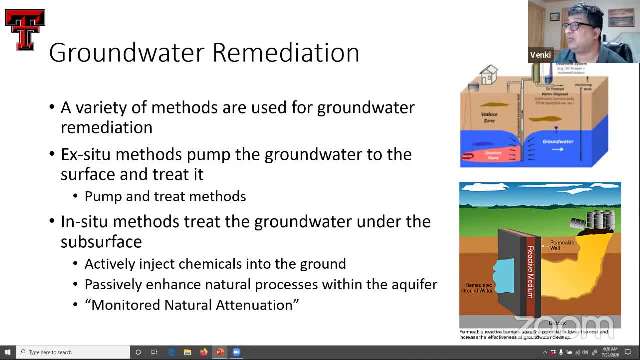 And, of course, the last part is what's called as the monitored natural regeneration, where we have to do a lot of things. We just monitor to make sure that our plume is stable, things are going down, but we are not doing any active remediation. 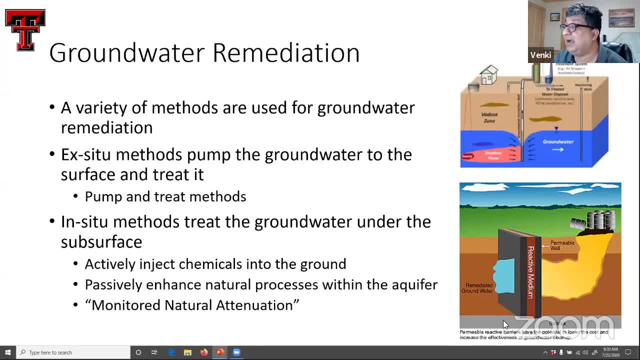 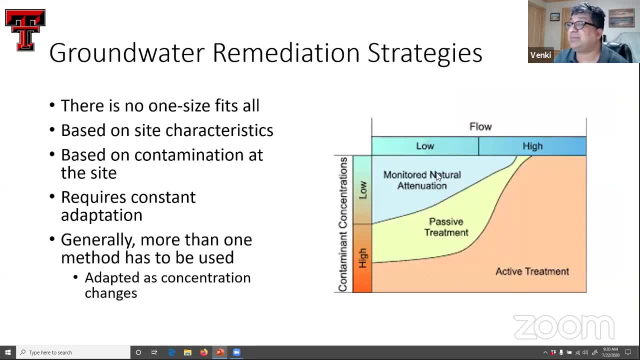 At best we are enhancing the microbes that are there in the subsurface and help them help clean up the remediation. So those are the three types of remediation that we do. If you have very high flows, very high concentrations, we have to do some active treatment. 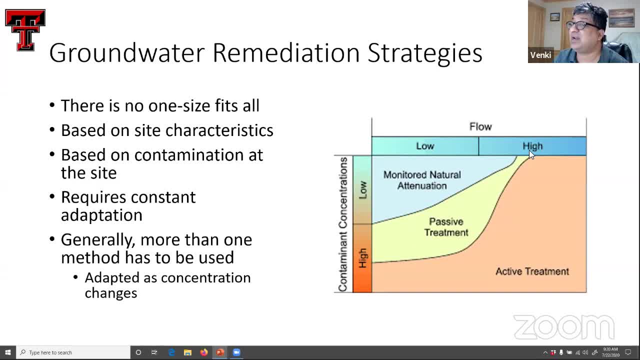 If you have reasonably high flows but high concentrations, sometimes we can do this passive treatment And then, under low flow, low concentration conditions, we end up getting to this monitored natural regeneration, which is usually the last step of our regeneration. So we start with active treatment and tend to go in that direction. 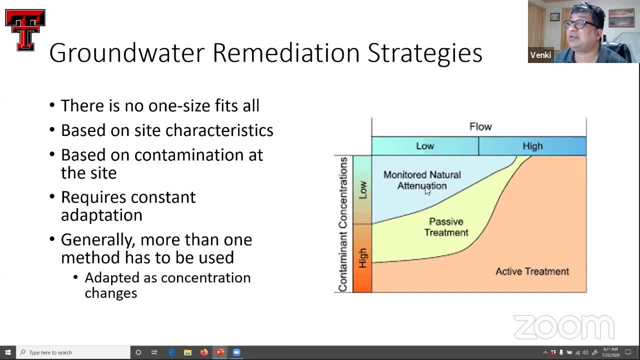 But a lot of times we can mix and match as well. We might be doing monitored natural regeneration, but occasionally doing some pump and treat when we want water. So generally we have to use more than one method. There is no one size fits all. 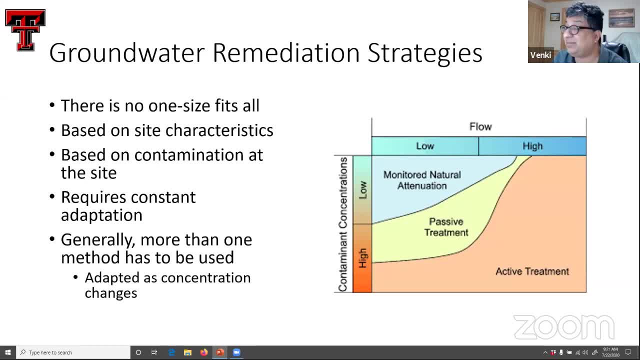 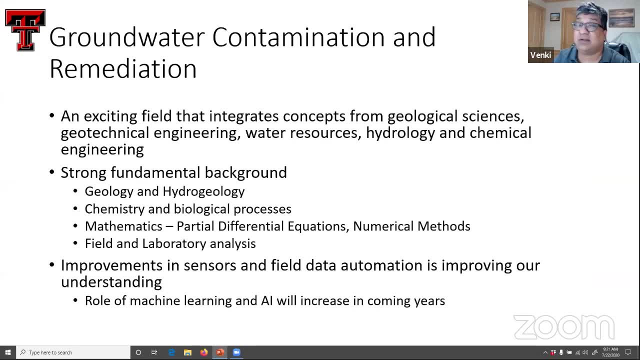 There is no panacea, no silver bullet when it comes to remediation. A lot of it is trial and error, because we are dealing with a lot of uncertainties and heterogeneities. So just to give you- that was a very broad overview of groundwater contamination. 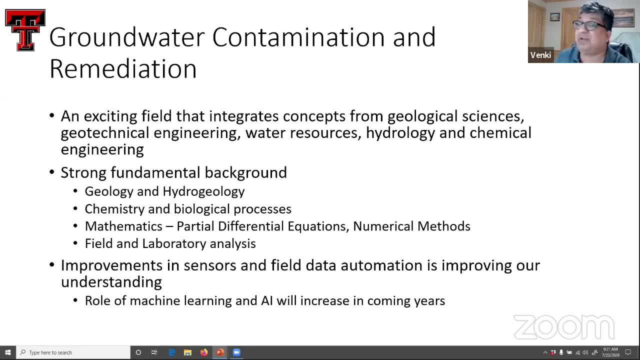 the modeling that we do and the type of data that we collect and some of the remediation techniques that we use. It's a very exciting field, especially if you like integrated interdisciplinary research. You have to integrate concepts from geological sciences, geotechnical engineering, water resources, hydrology, chemical engineering. 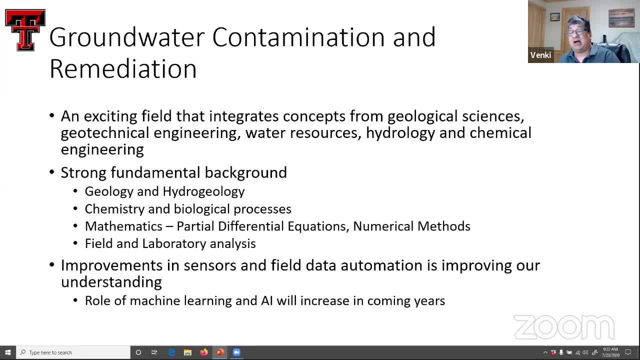 So we use concepts from broad variety of fields. toxicology: sometimes you know to come up with knowing how to clean up. So if you're interested in this field as students, I strongly recommend you to get something like this. You have a good background in geology, hydrogeology. 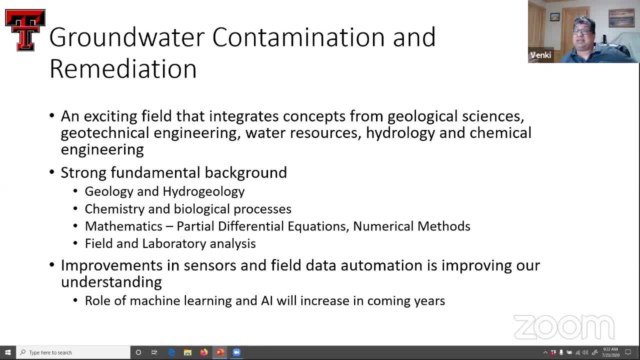 Brush up your chemistry, your freshman chemistry, mathematics- especially partial differential equations, numerical methods, And then have a good understanding of field surveying and field methods and laboratory analysis. So, as you can see, we use models, we use field data collection and laboratory analysis in conjunction to solve these problems. 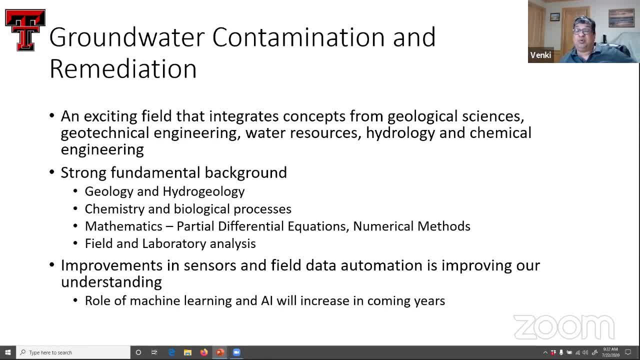 One of the things that's happening is the sensors have improved quite a bit, And so that is helping us do a lot of field data automation, which means we are collecting a lot of data, a lot more than what we did historically. So now we are exploring tools like machine learning and artificial intelligence and big data methods to solve these problems. 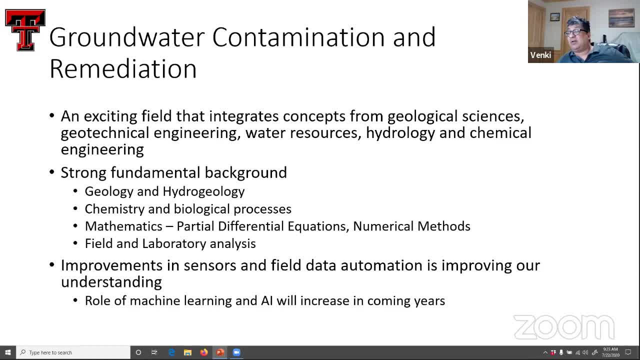 to solve and develop contaminant transport problems. So that's another exciting field where we are integrating artificial intelligence and machine learning to solve groundwater contamination problems. So that's a broad overview of this field. So I'm going to stop here. Thank you all for your time. 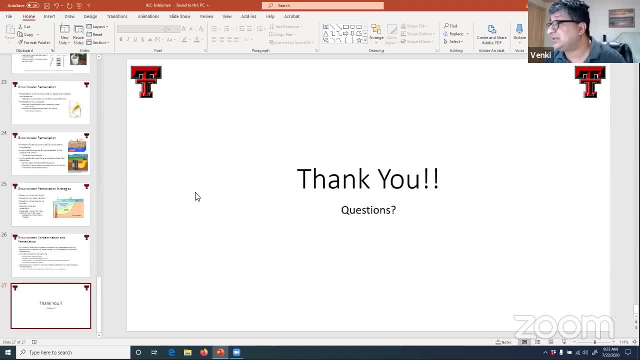 And then we'll take any questions, And I think we have a few minutes left for Q&A, So are there any questions at this point? I'm unable to see the chat box, so I'm not sure. Thank you, sir. Thank you for valuable information. 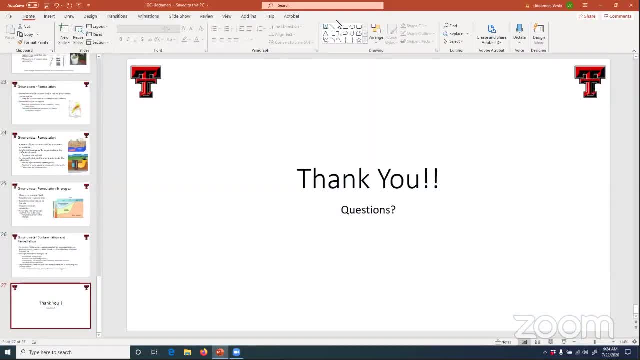 And valuable information sharing to all the participants. Before question and answers, I'm sharing the feedback link to all the participants. Please, all of you give your feedback regarding the webinar lecture. After that, please, all of you ask your question and answer questions through chat mode only. 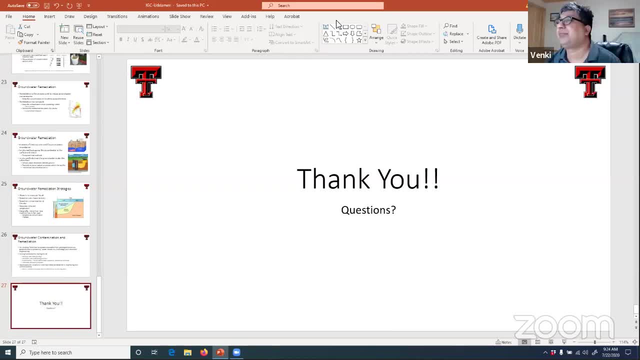 Sir Uddamuri. sir, Yeah, Please see your chat box, sir. Yes, yes, sir, All the audience are asking questions. Okay, I have the chat box open, but I don't see any Participants. just now I shared the feedback link to all the participants. 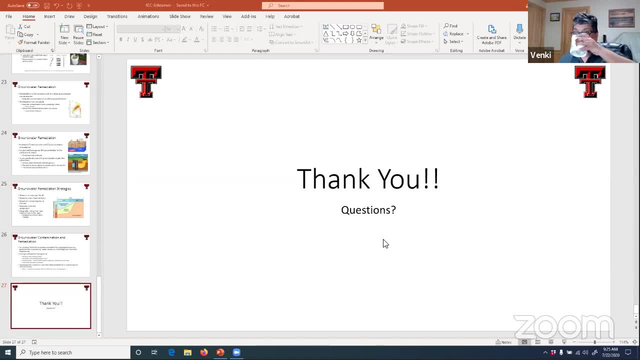 Yes, I saw that. So please, all of you give your valuable feedback And ask the questions to today's speaker, Uddamuri sir. So please, all the participants, ask your questions. All the attendees, do give your feedback via the chat box. 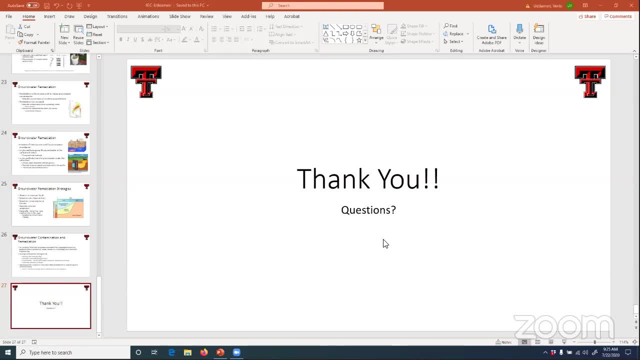 And this is the participation itself. So, please, all of you, give your feedback. Thank you, Thank you, sir. Okay, Thank you all. all of you, All of you give your feedback, raise your hands, jump right, the dot. 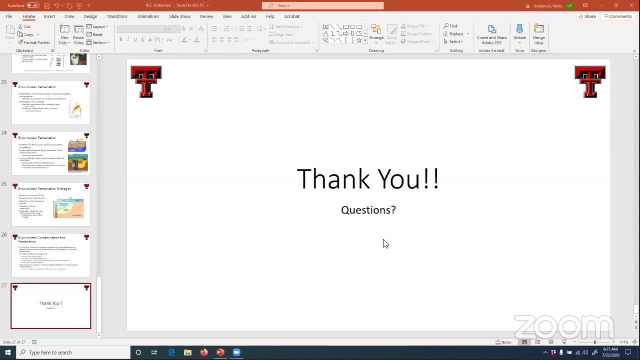 Awesome. thank you all of you. Yes, you now have 30 seconds to answer all of your questions. So Kiran Kumar asked a question about hasゃ. has any non-destructive or geophysical investigations used for determination of contamination of groundwater? that's a really good question. 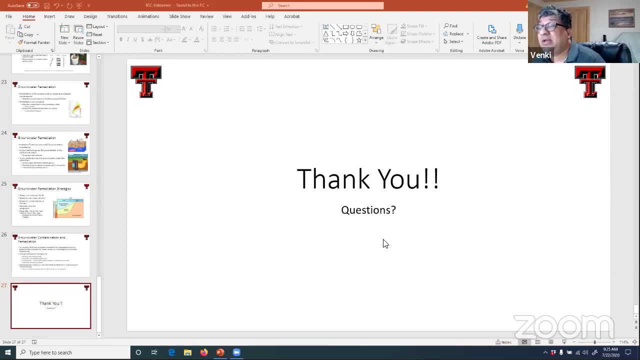 non-destructive geophysical investigations. we do use some of some of them but it tends to be a little bit challenging because a lot of times the contaminated sites, especially that in urban area, they are very difficult. you know you get a lot of interferences with the non-destructive testing method. so there is a lot of interest in using. 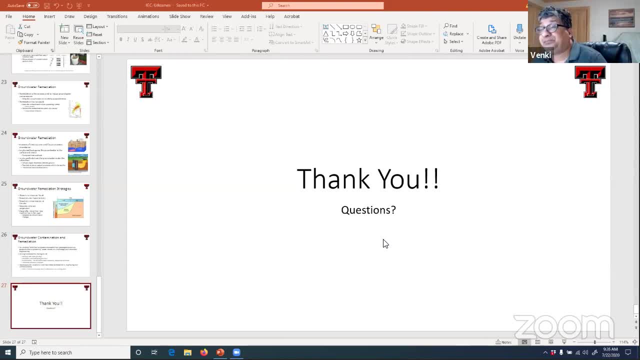 non-destructive testing methods, but a lot of times their usage becomes limited because of the interferences that you're going to get. the deeper formations tend to do very well with geophysical investigations, like you know so, but when we deal with shallow subsurface, non-destructive methods are a little bit. 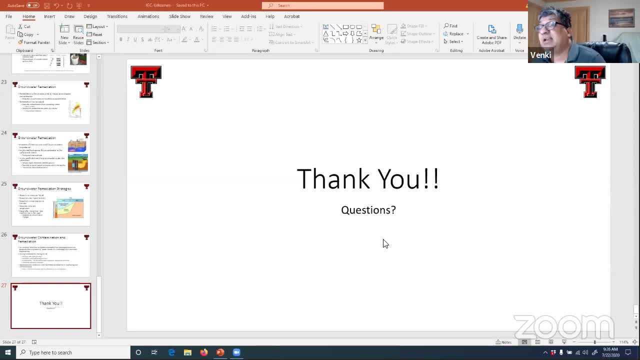 difficult because of the interferences we're going to get with other structures and other things that are going on. so that's the answer. so people are talking about COVID-19, biodegradation in water body. is it investigated in any part of the world? yes, a lot of people are. 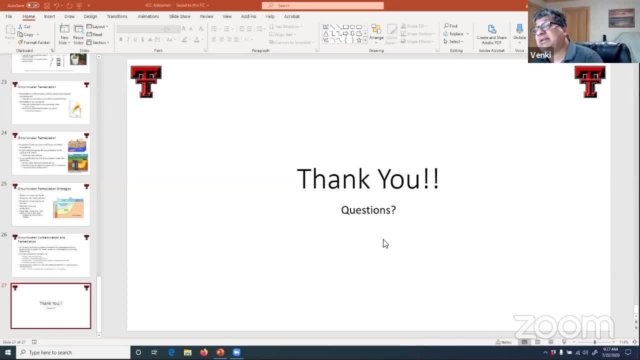 looking at. one of the things about COVID-19 is that COVID-19 can affect your lungs- we all know that- but it can also affect your intestines. there are sites on your intestines- large intestine that- that the virus can actually bind to. so so you don't see COVID-19 in urine samples, but you do. 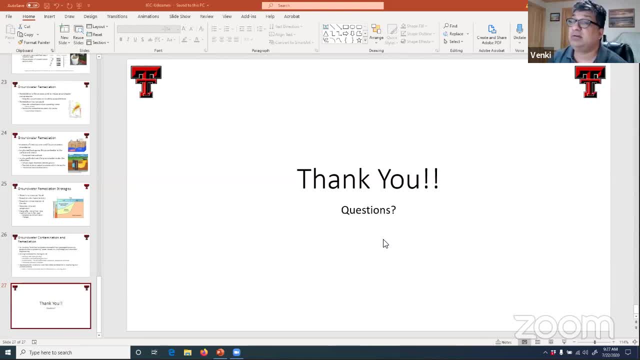 see them in stool samples and people are trying to use waste water. they have not really seen active COVID-19 virus yet, but they have seen filaments of COVID-19 virus, because the COVID-19 virus is not as strong as an enteric virus. you know, the enteric viruses are what are in your gut. 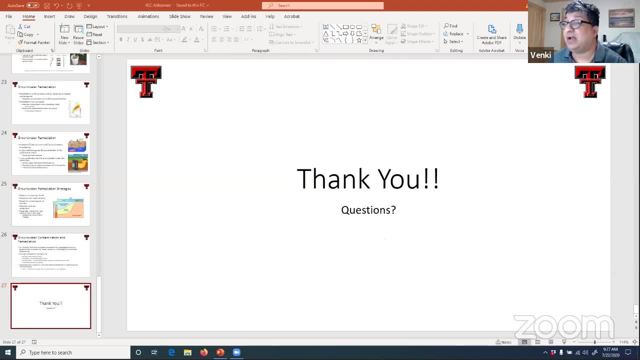 they pass through your digestive system so they're very, very robust. so you will see them in waste water or even in groundwater systems. but, COVID-19, you're seeing trace filaments and things like that. so people are trying to use that to say: is there community transmission, and things like that. 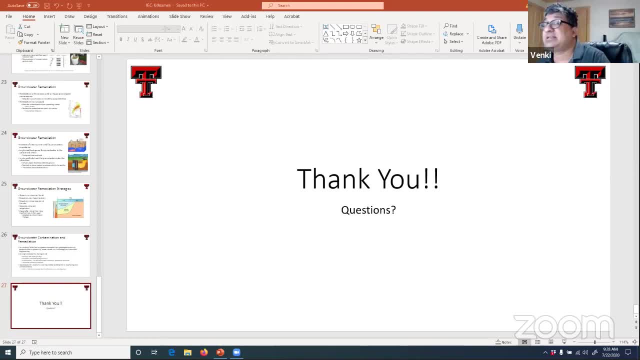 so that's what people are using. another question is: is there any modern techniques available for improving groundwater tables, methods for reducing the groundwater contamination? again, a very good question. we do a lot of recharge- artificial recharge- to improve groundwater tables, but they tend to be difficult because they clog up or like they use up land space. 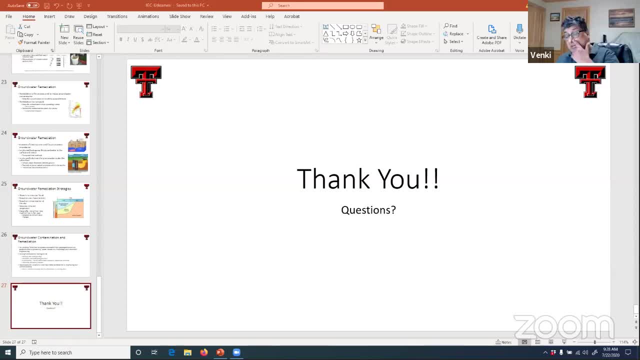 so, particularly in developed countries, in like Texas in particular, there is a big push to go towards deep one injections, as opposed to creating open pits and then find the percolate water. so in terms of reducing groundwater contamination, really it's education and people not disposing of, you know, waste improperly. that's, that's the biggest, that's. 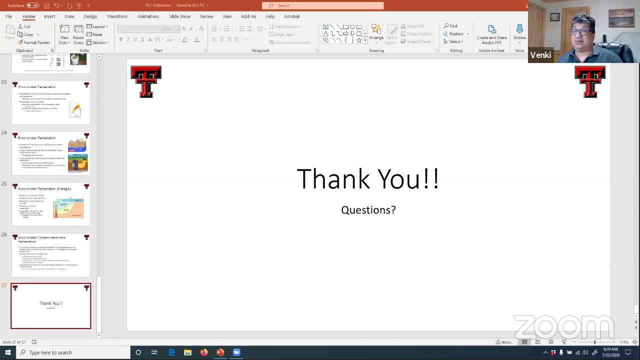 the biggest challenge. so a combination of education and enforcement is typically what's used to improve water quality, so that we are not disposing our waste chemically. what kind of chemicals to be injected for groundwater treatment would you suggest? that would really depend on the contaminant of interest to us if you're dealing with organics which can biodegrade. typically we put in oxygen. if you have a deeper aquifer and we know that there are cellophane reducing bacteria or you know methane reducing bacteria, we try to put those types of things. so that's, and again, if we, if you're, if you're dealing with things like institute treatment, 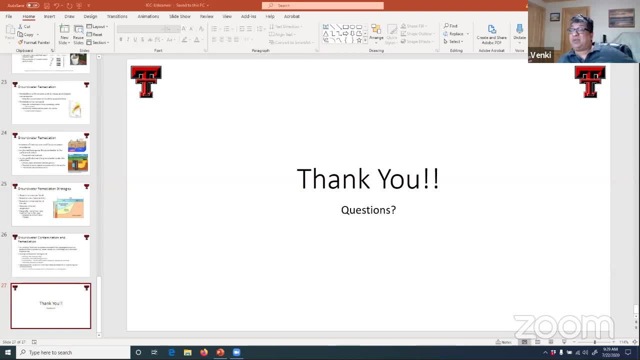 of fluoride and arsenic, which is another question. arsenic is a very interesting compound because arsenic is mobile both during, in a reduced form, as well as in the oxidized form, which makes it very, very challenging to treat arsenic in this way. the second question is: what is the best way to treat arsenic? 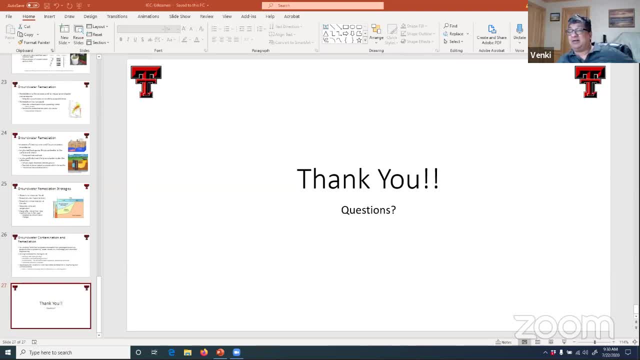 in situ In terms of fluoride and arsenic. typically we want to change the redox condition, So we can do it either using microbes enhancing the microbes that are there, but abiotic reactions can also take place, but they are very difficult to do over large areas. 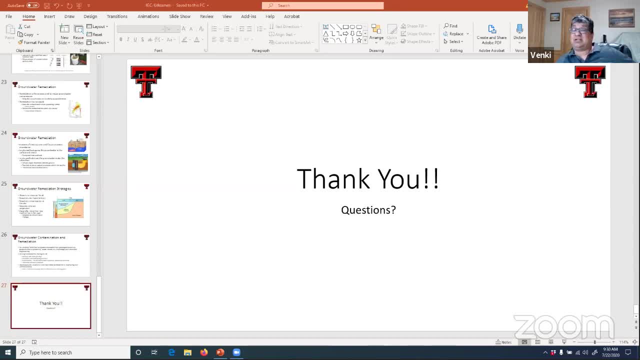 So the in situ treatment techniques for fluoride and arsenic generally are to change your redox conditions and that are facilitated by putting organic substances, nutrients and pH control. Can you please elaborate on the role of artificial intelligence in this field? in the field of remediation? Yes, the field of artificial intelligence, so we use neural network type models. 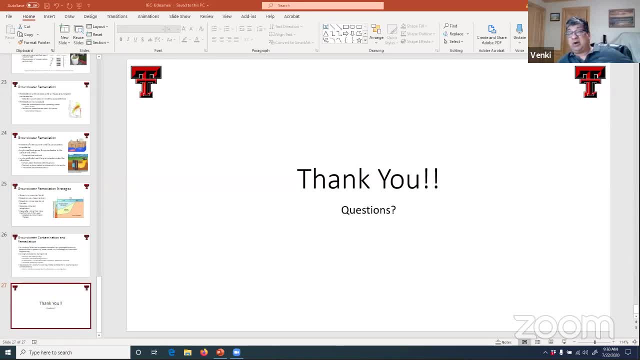 to develop predictive models to forecast what the concentrations are going to be at different wells and different temperatures. So we use our mediation to predict what the concentrations are going to be at different wells and different temperatures. So we use our mediation to predict what the concentrations are going to be at different wells. We're using artificial intelligence. 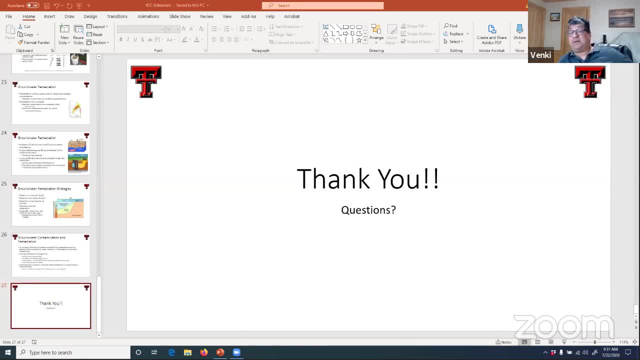 techniques to do better mapping of our plumes from scarce data sets. We're using fuzzy logic, for example, which is a way to capture decision maker preferences, because when it comes to cleanup of sites, somebody will say: I want to bring it down to drinking water level, Somebody 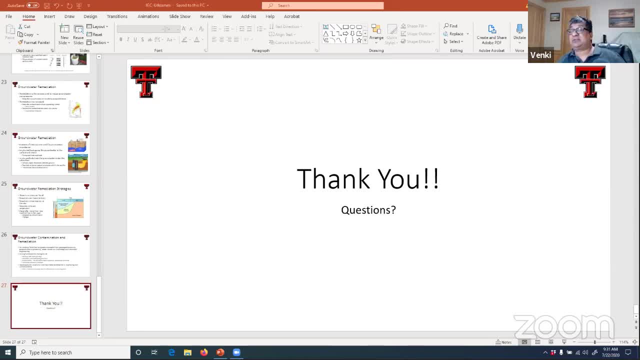 will say: well, we don't need to do it to that level, We can use it for some other purpose. So there would be conflicts among decision makers. So fuzzy logic gives us a way to capture that. There are tree-based models that we have developed: regression trees, random forest type. 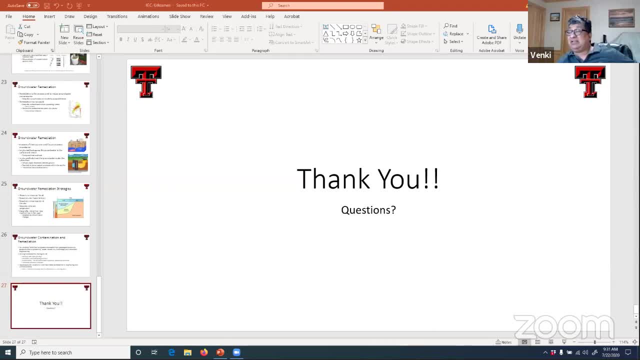 models. The tree-based models, are very easy to explain to people because you get a tree and you say, well, this affects this, and also to mine data and get cause and effect relationships that can be used to guide our field sampling methods. In addition, we are using cloud quite a bit to collect data remotely, So cloud 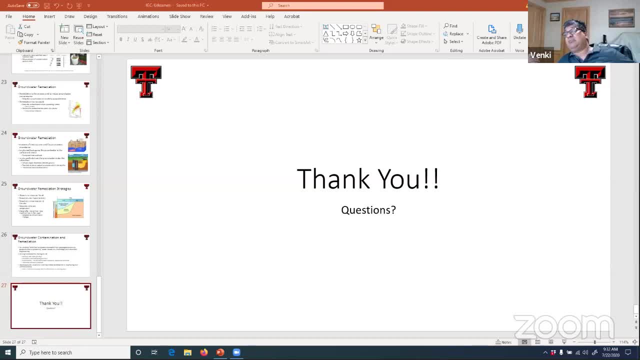 services, where data goes into a cloud and then we can pull it out and put it into our models. So that's another area where you're seeing a lot of AI being used. We're using edge computing, which is doing some calculation at the sensor level itself. Can we use groundwater contamination? 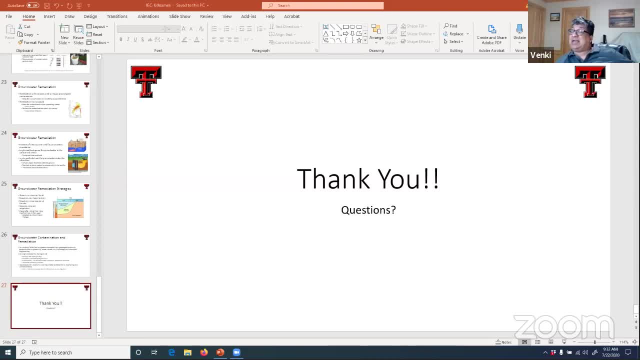 with help of satellite imagery, Not as easy as finding surface water contamination, because this is a very complex area. But it's not as easy as finding surface water contamination because this is a very complex area. But it's not as easy as finding surface water contamination because this 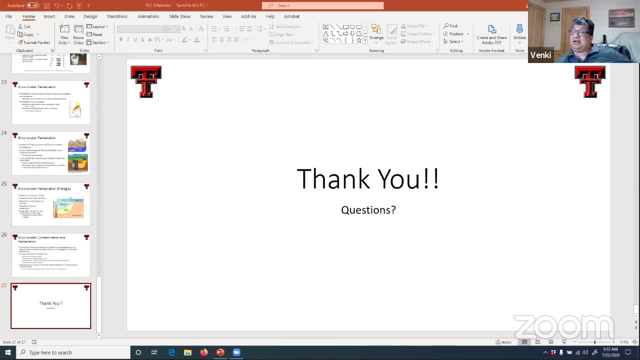 is deep And we don't have satellites that can capture what is happening at that sub-surface depth. But satellite imagery sometimes can give us a good idea of the sources of contamination. So what's happening on the surface can eventually tell what's the likely source. So we do use 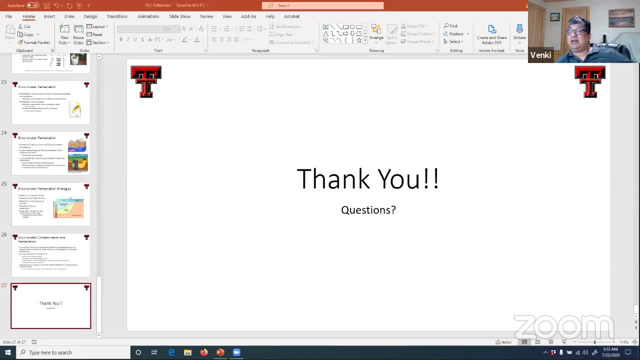 satellite imagery, but not directly contamination, but indirectly. So is there contamination due to aquaculture? Yes, aquaculture actually. So when you grow shrimp or when you go fresh, there is a lot of fecal matter that comes out. The fish are fed with proteins, the food products 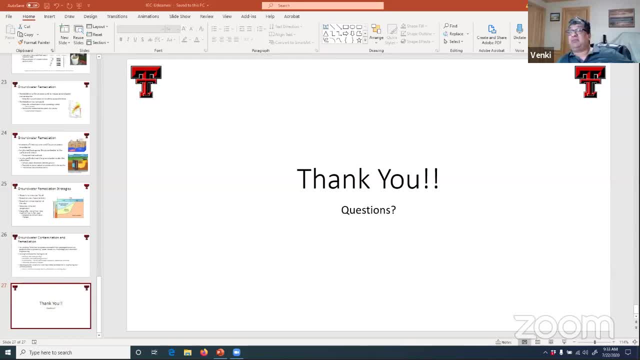 So there is a lot of BOD, COD type, and then the nitrogen-based contamination that's associated with aquaculture. A lot of places it's not regulated. Texas is one of those places where it's used. Ashish is asking. thank you, sir, for your lecture. 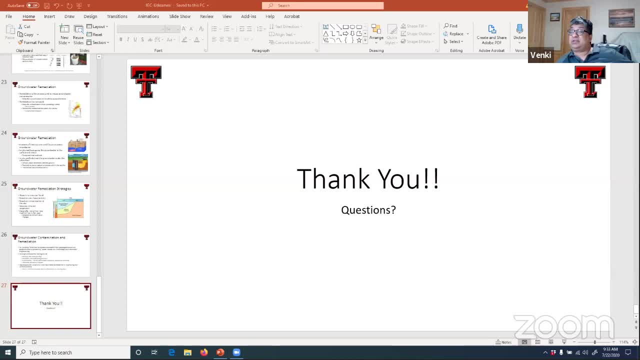 Is it possible to use ancient techniques such as Persian squanauts to bring water from distant sources to the contaminated areas? Yes, we do bring water from different sources. The canards or the flood systems work very well in certain types of formations. We can't really do. 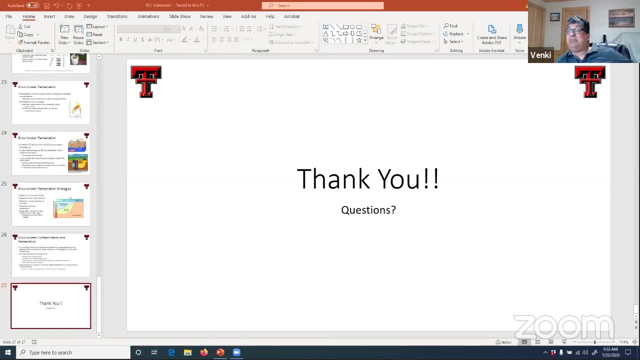 that in sand and gravel aquifers. But if you have deep bedrock aquifers we can move water. But again, that's possible, It's used. It's a question of economics. Doing something like that in today's day costs a. 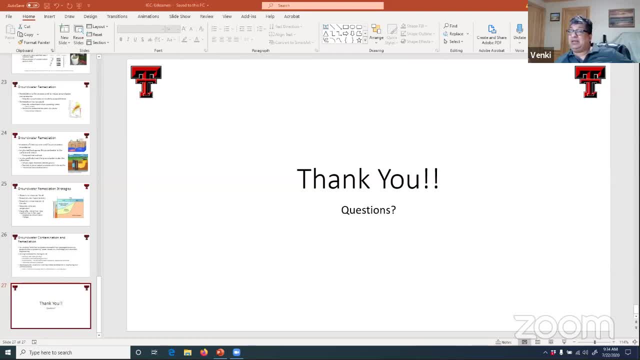 lot of money and that would be difficult. Could you please brief about the impact of mining on groundwater in terms of quantity and quality? Mining usually creates acid, mine drainage or other types of metals- heavy metals- So when they get into the contaminator and they get into groundwater, redox drives a lot of those. 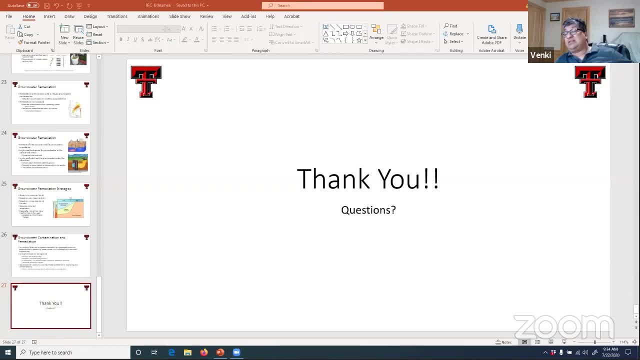 reactions So they change the redox to groundwater, which can change the microbes which can then affect your water quality. In terms of groundwater use, groundwater use is quite developed. especially if you do open cast mines and other things, People use groundwater.